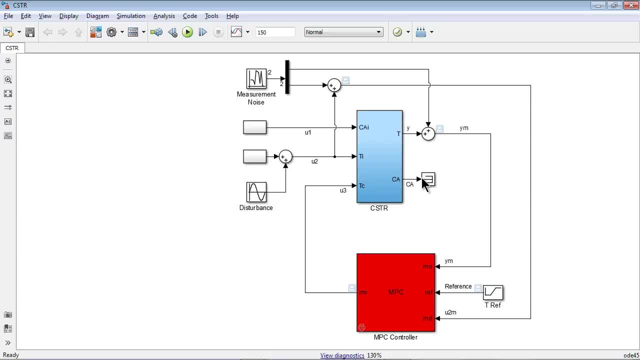 Plant has two outputs. The second output is not really the same, It is not really something that we are interested in- But the first output is temperature signal Y. here We are adding some measurement noise to make the simulation realistic And that is what we feed to our controller to close the feedback loop. 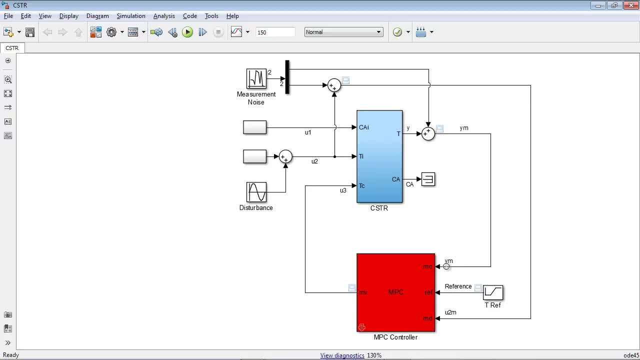 Our controller also receives a reference signal that we want the temperature to follow, And it knows about the disturbance because in this case we can measure it. So it is using some feed forward control to reject it. Now the reference profile for the temperature is a ramp from low value to a higher value. 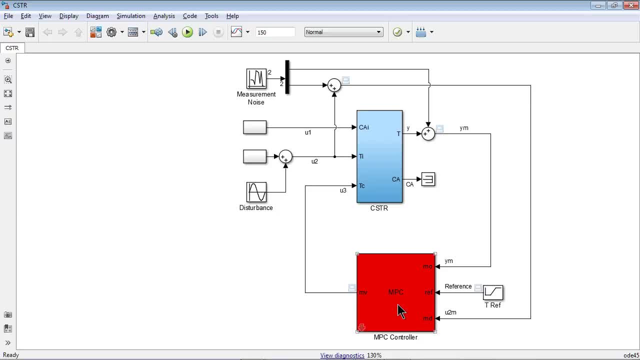 In this case, we start with a controller that is not an adaptive controller. It is a more traditional controller that is designed at a single operating condition, specifically at a low temperature- the initial value that our reference starts from, Because the plant dynamics is changing quite significantly during the transient. 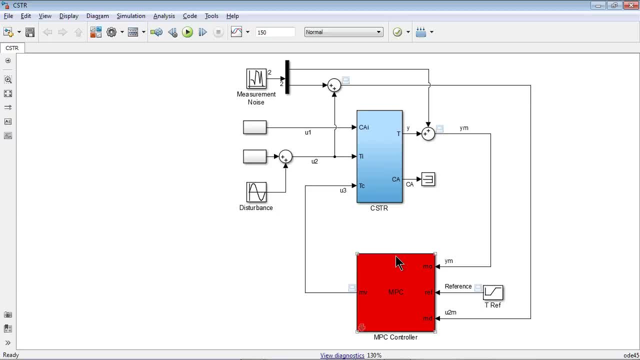 this controller designed at a low temperature- the initial value that our reference starts from- Because the plant dynamics is changing quite significantly during the transient, this controller designed at a single operating condition cannot effectively deal with significant changes in plant dynamics. Let's run the simulation to see that. 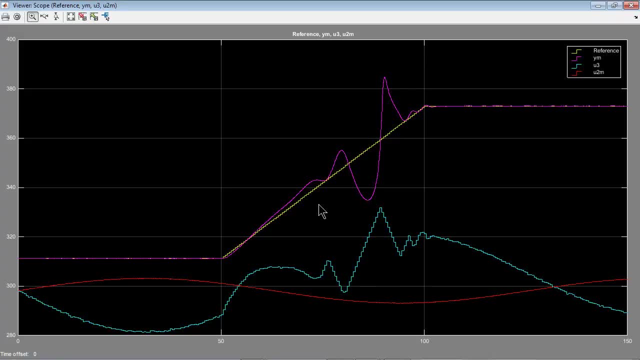 Let's look at the results. Here we see a few lines. The yellow line is the reference trajectory for the temperature. As I mentioned, it starts from a lower value and ramps up to a higher value. The magenta line is the measured temperature. 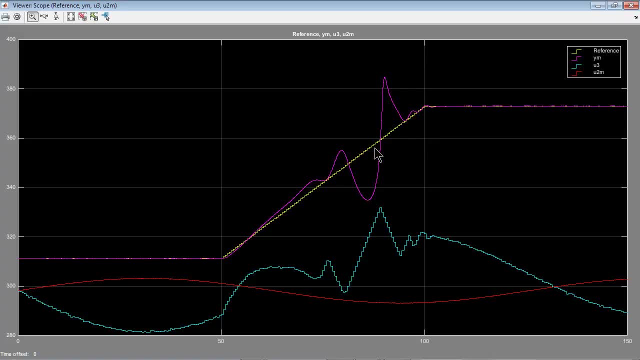 As we can see here, our controller is not doing a good job in tracking the reference signal, And this is happening because the plant dynamics is changing significantly during the transient. In fact, in this operating region the plant is unstable. The cyan line that we see here is the manipulated variable, the value that controller commands. 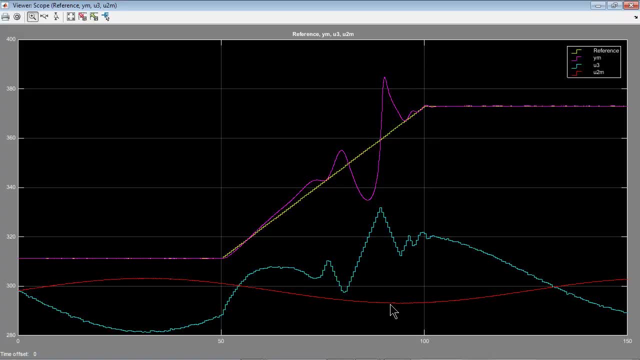 And the red line is the measured disturbance. So, as we see, the controller designed at a single operating point is not very efficient. Of course you could try designing a controller at a different operating point, for example, the higher the final value of temperature. 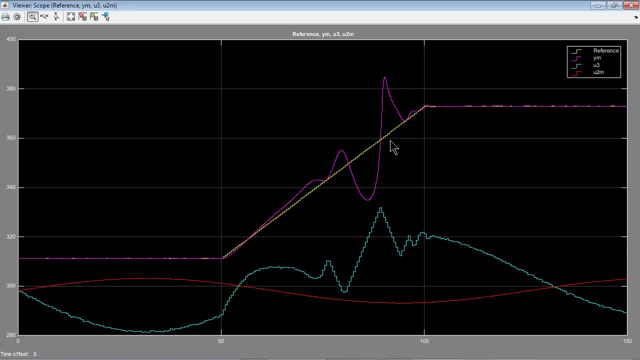 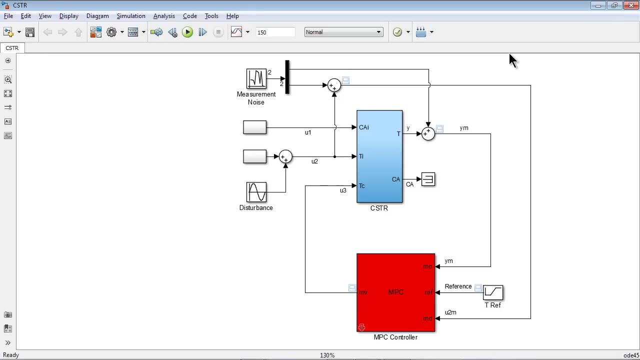 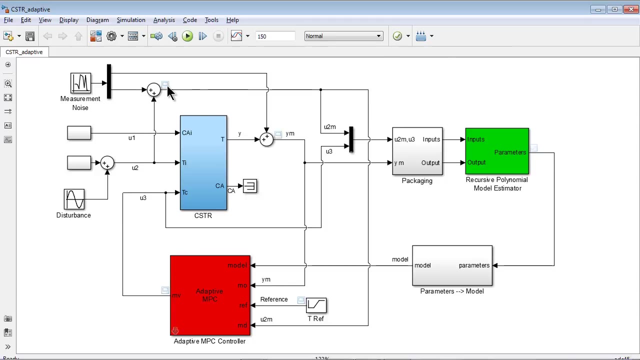 But if you try to do that, you will see that still, it wouldn't provide a good performance during this transition. So let's now look at a different model where we implemented an adaptive controller. Here is that model. You see that the blocks on the left look very similar to the model we just looked at. 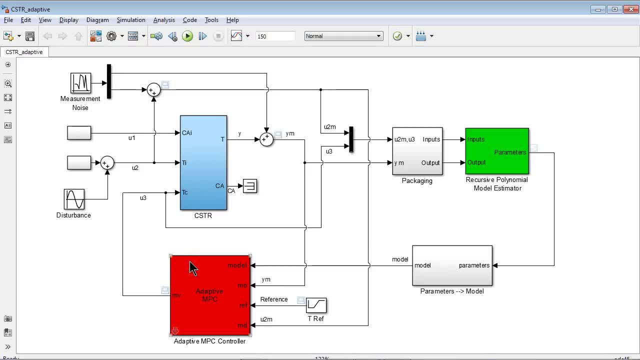 We still have a plant model with three inputs. We have the controller block, But the one difference that you will notice in the controller block is that, in addition to the measured temperature reference signal and measured disturbance, it has one extra input for the model. 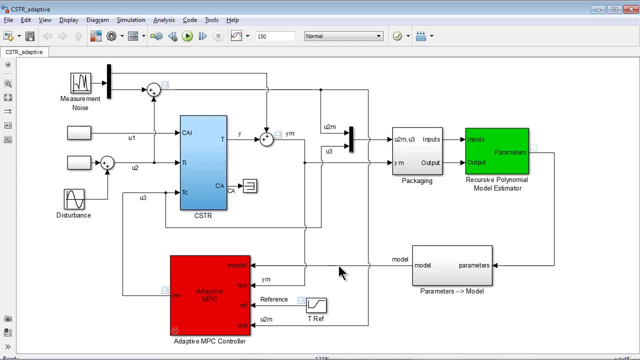 Now, this model that we estimate online comes from primarily this green block here. So let's look at the image. We have inputs and outputs of this green block, So the inputs are basically plant inputs and outputs. So that's what you see here. 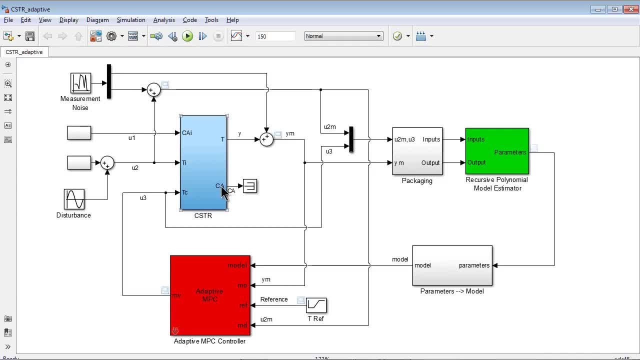 Inputs and outputs. In our case, plant inputs that we are measuring are the manipulated variable U3 and the measured disturbance U2M. So the two signals here, And the plant output is the measured output YM. So that's the signal that you see here. 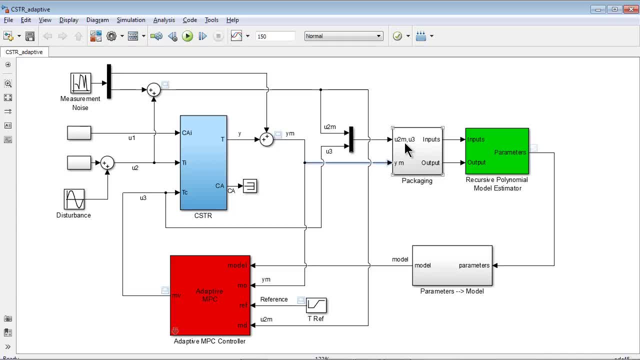 We do some packaging and data manipulation with those signals And we pass them to this block that performs online parameter estimation Using plant inputs and the plant output- in this case, again, two inputs and one output. this block comes up with parameters that describe how the dynamics of the plant is changing. 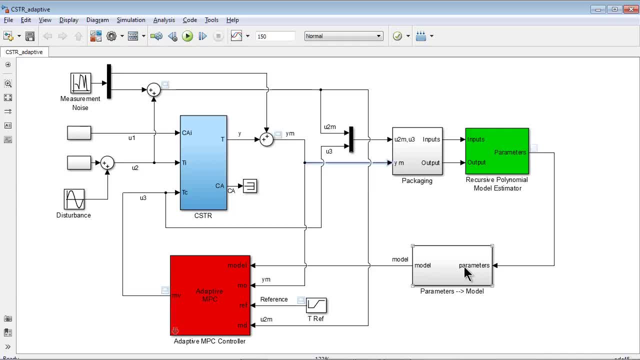 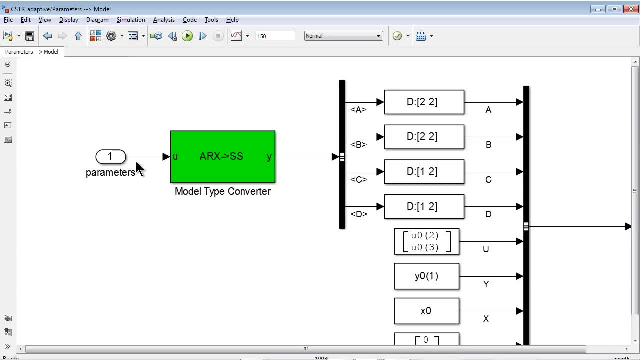 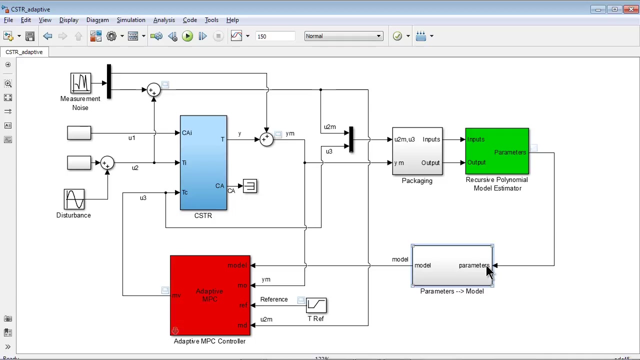 We then do some additional manipulations with those parameters. If you look here we convert the parameters that come from the block that we saw at the previous view into a state space system. So that's what model type converter block does here. So we are estimating some parameters here, converting them into a state space system form. 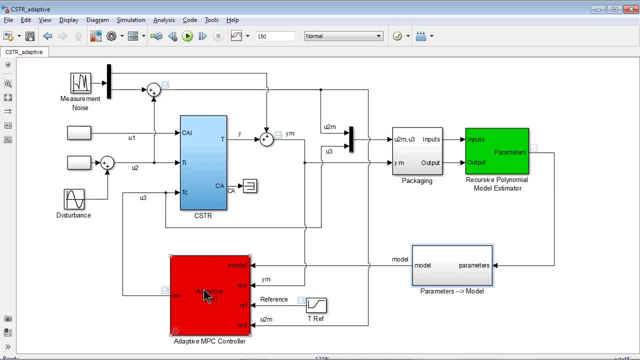 And that's the model that we feed to our controller. Now our controller is using this model that is changing at runtime To adjust controller behavior dynamically. So let's see how this works. We will run the simulation. We will look at the simulation results. 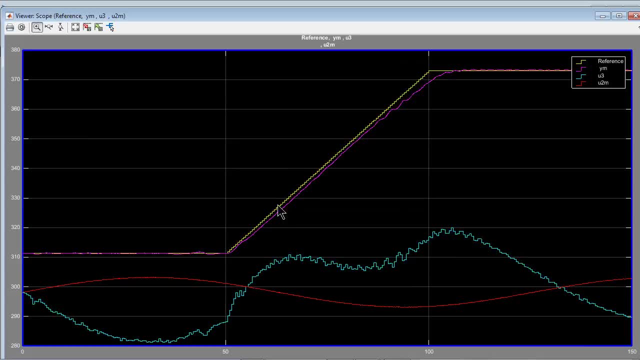 Again, the yellow line is the reference trajectory, the same profile as in the previous model, But now the magenta line, which is the actual measured temperature, looks much, much better. So reference tracking is indeed much improved And again, the sign is manipulated variable and we have exactly the same measured disturbance profile. 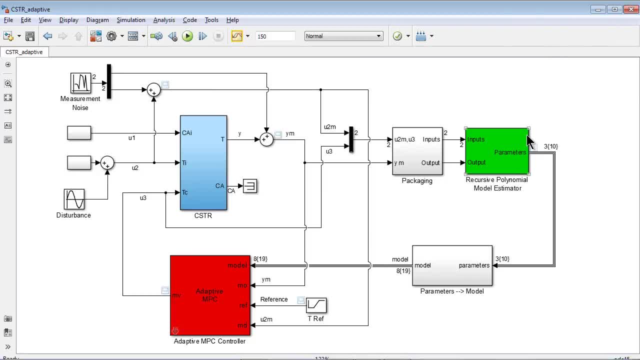 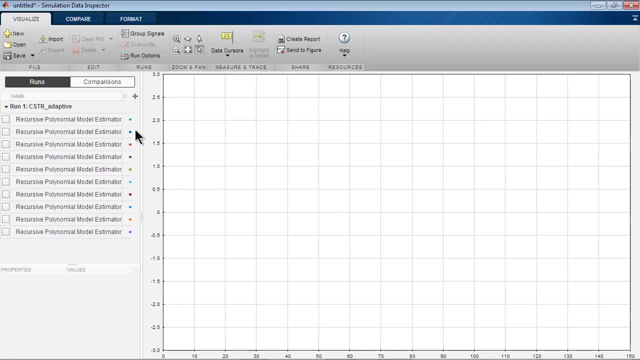 In addition to this plot, I also recorded the parameters of the plant that are coming from this block that is doing online parameter estimation. Let me open simulation data inspector to take a look at some of those parameters. Here we will see various different parameters that we are estimating. 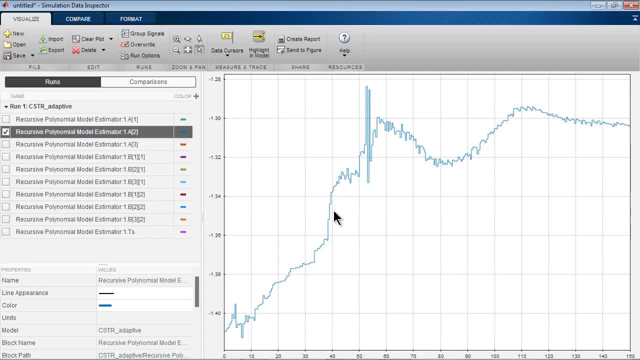 And if you look at some of them, you will see that they are changing during the simulation And so these changes, basically are capturing changes in plant dynamics and are letting us to adjust controller behavior dynamically during operation of the plant to provide good reference tracking. 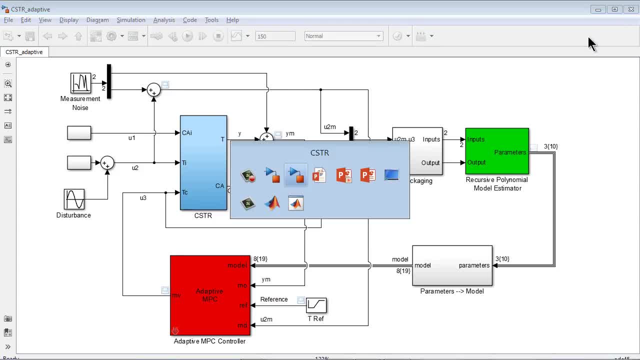 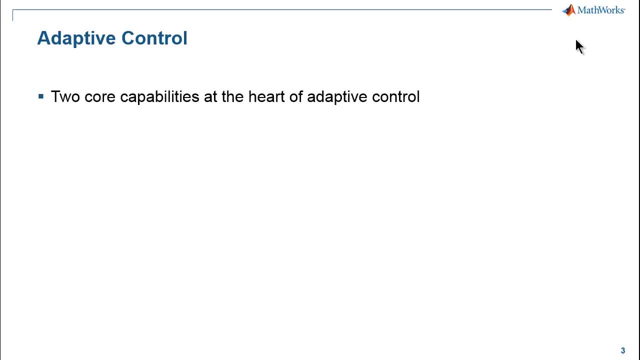 Now let's go back to the presentation. Let's step back for a second and talk about what adaptive control is. At the heart of any adaptive controller. there are two core capabilities, And we saw them in our example. One capability is online parameter estimation. 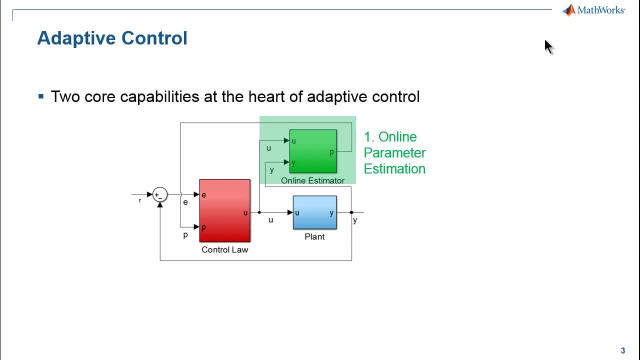 You need to be able to detect how plant dynamics is changing online. And once you know how plant dynamics is changing, you need to be able to adjust controller behavior to adapt to the changes in plant dynamics. And that is done by the control wall that can adapt to the changes. 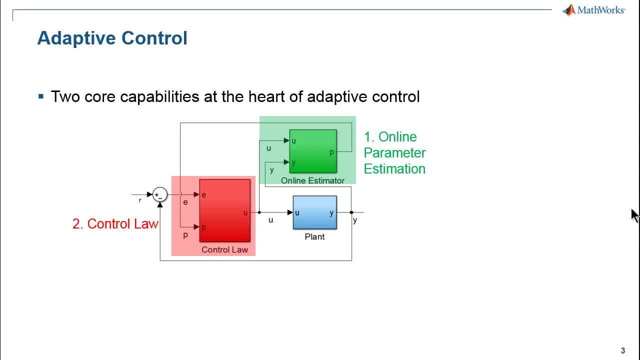 So again, you see here in this diagram that the online estimator gets plant input U and plant outputs Y and produces parameter values that describe how the plant dynamics is changing. Now the controller, in addition to getting the error signal between the reference and the measurement, 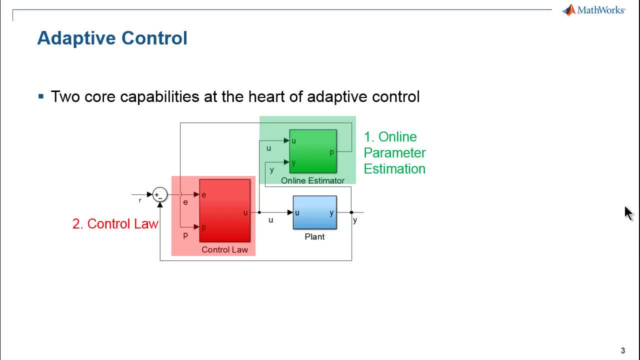 is also getting those parameter values from online estimator and is using those parameter values to adjust how it computes the manipulated variable or variables U. So in the webinar today we will talk in quite a bit of detail about these two capabilities: online parameter estimation and adaptive control wall. 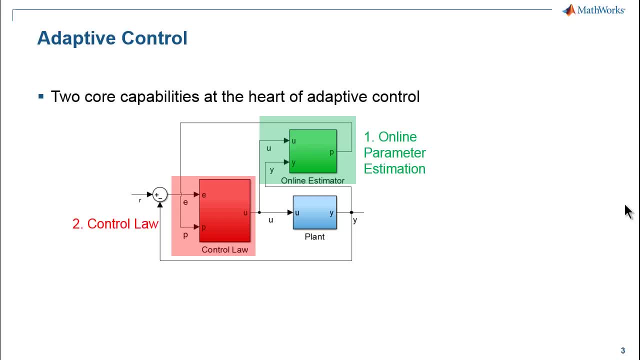 Arda will talk about online parameter estimation and Ron will show you how you can develop an adaptive controller. Now it should be said that there are many approaches that can be taken to design an adaptive controller. Gain scheduling is a very common example of an adaptive control. 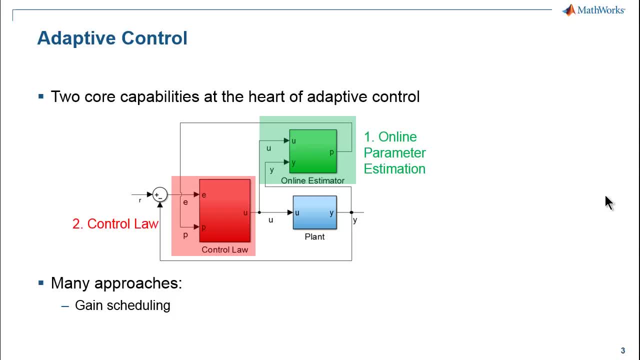 where you detect changes in the operating condition and you schedule controller gains according to how the operating condition is changing. There are also other schemes, such as small reference adaptive systems and many, many other schemes out there as well. Now, today, in this webinar, we are not trying to give a comprehensive overview of all the different ways to implement adaptive controllers. 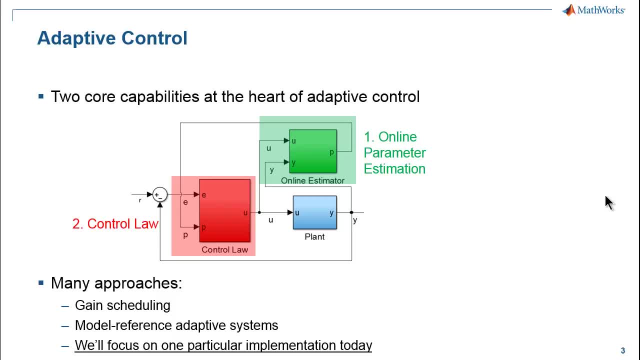 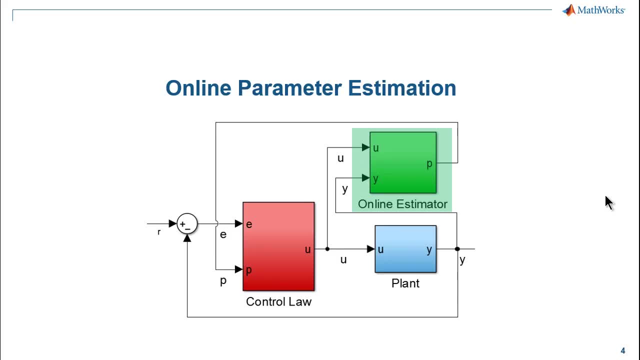 We just want to focus on one particular implementation that is available out of the box with the capabilities that we currently ship in our products. So with that, let's start with talking about online parameter estimation capabilities, and I'll invite my colleague, Arda Ozdemir. 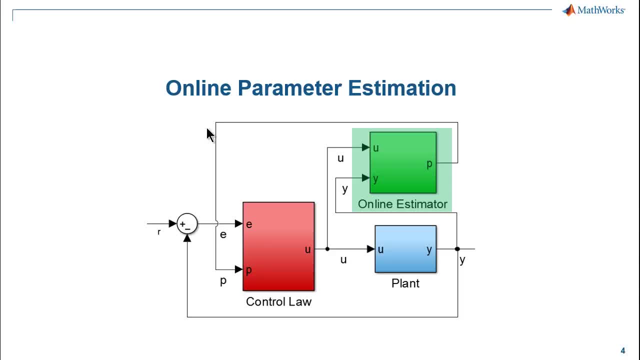 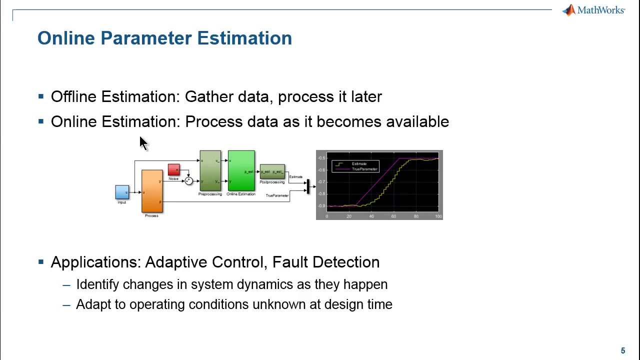 to start talking about that, Arda? Hello everyone, I'm Arda Ozdemir and I will give you a little more details about the online parameter estimation capabilities we have today. Some of you may be more familiar with offline parameter estimation and offline system identification. 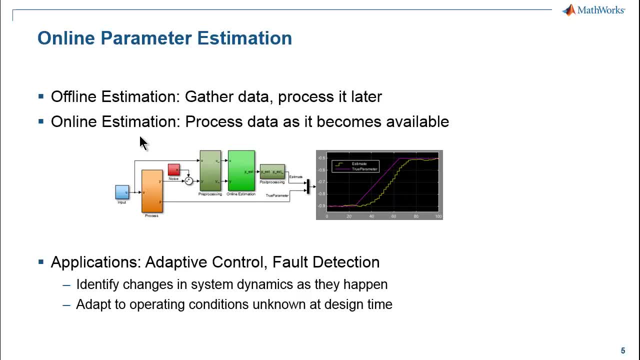 Therefore, I would like to start with a comparison of online and offline estimation. Offline estimation is where you just run your process, gather your data, log it and then you go back to your PC or tablet and process the data later to come up with parameters or your system model. 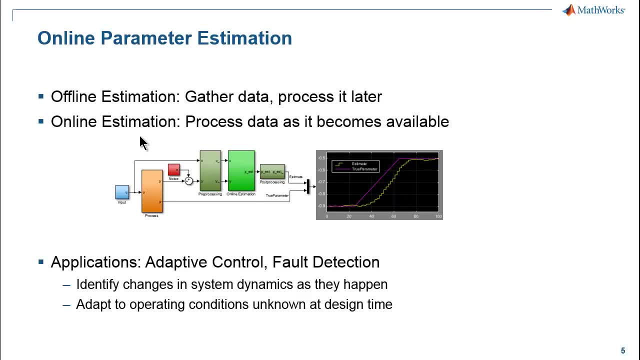 In contrast, in online estimation, what you do is you process your data as it becomes available while your system is operating, typically using the processors that are embedded on your system. Here in this block diagram on the left, we see a very typical implementation of online estimation. 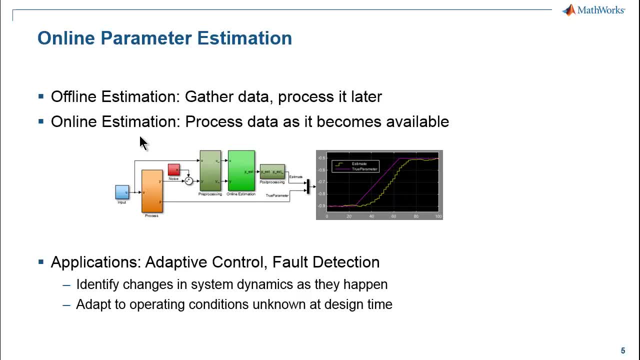 In orange you may have your process that you are interested in observing, whose dynamics will be changing over time, and then you take its input and output signals. you take these measurements and then do some pre-processing, just like in offline estimation. 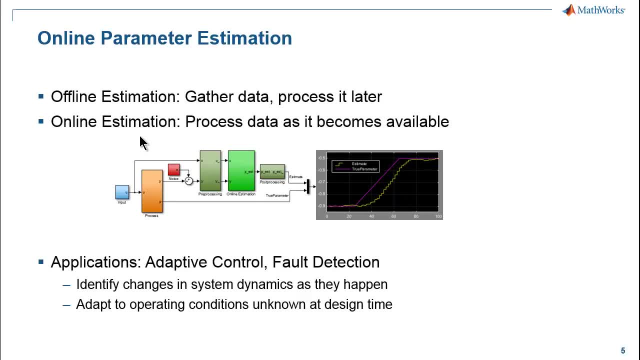 This step may consist of removing some outliers, removing sensor biases, removing trim conditions. After you pre-process these signals, you would feed these into your online estimation algorithm and then after that, for example, you may have a post-processing step where you may be validating your estimated parameters. 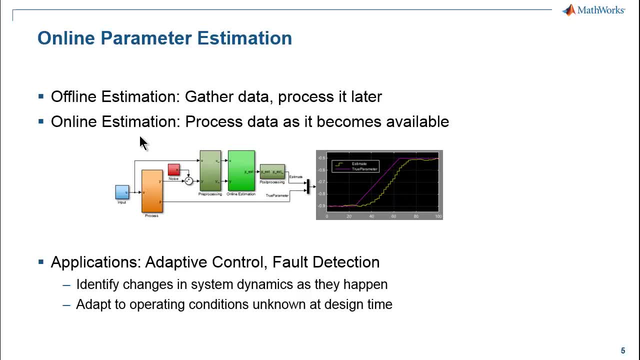 Most typical applications of online parameter estimation are adaptive control and fault detection. The main goal is identifying changes in the system dynamics as they are happening, and the main reason you would use online parameter estimation is to adapt operating conditions that are unknown at design time. 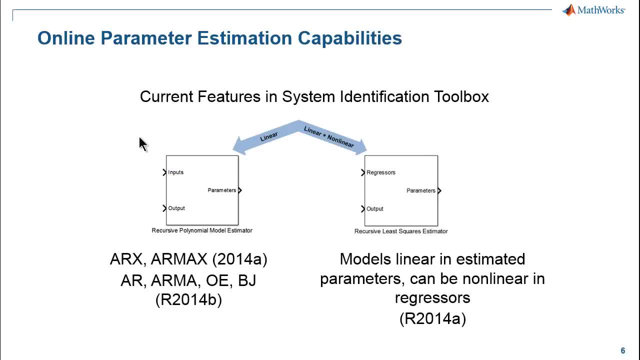 The current online parameter estimation capabilities we have in System Identification Toolbox consists of two blocks. The first one is so-called recursive polynomial estimator block. As the name implies, this block estimates linear polynomial models. These are ARX, ARMAX, AR, ARMA, OE and BJ. 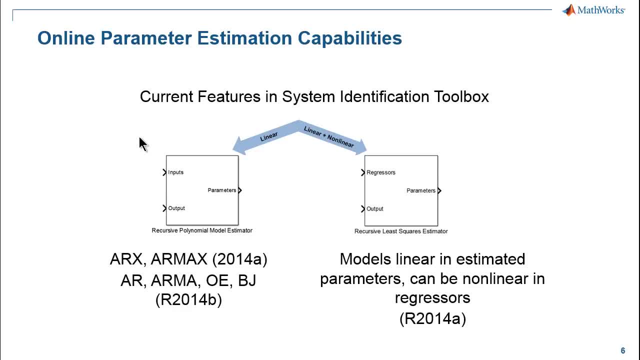 I will tell you a little more about these model structures in the next slide. Of these model structures, ARX and ARMAX models can be estimated with our 2014a release, and the other model structures are available in the 2014b release. 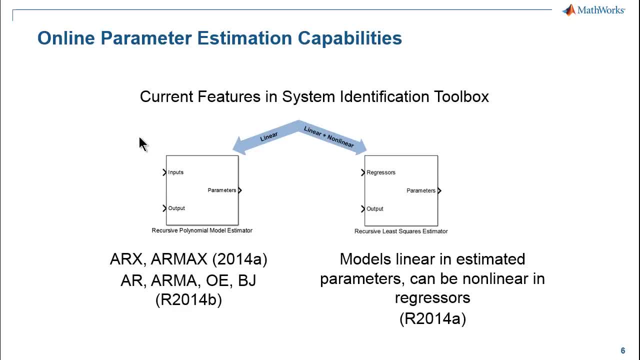 The second block we have is the recursively squares estimator block. This is a more general-purpose block which can be used for estimating any kind of models that are linear in estimated parameters. This basically implies that the model can be non-linear in its regressors. 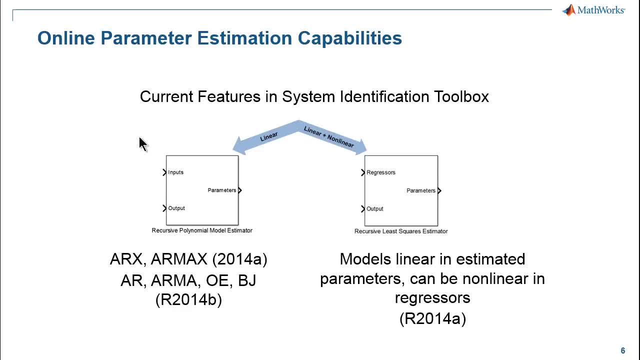 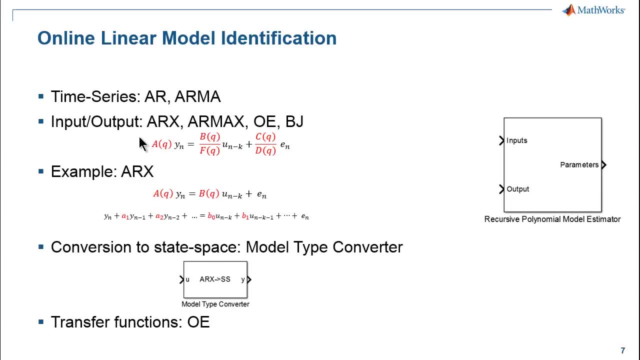 This block is available in our 2014a release as well. I would like to provide you a little more details about our recursive polynomial estimator block. First of all, we can divide the model structures estimated by this block into two categories. The first one is time series. 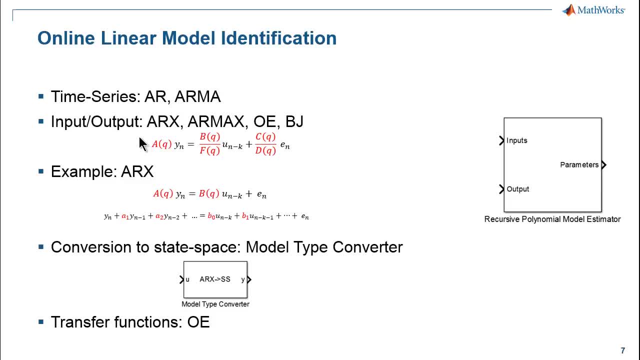 where you only have access to output measurements from your system. These model structures are AR and ARMA. The second type is so-called input-output models, where you have access to both input and output measurements from your system. These are ARX, ARMAX, output error and box Jenkins. 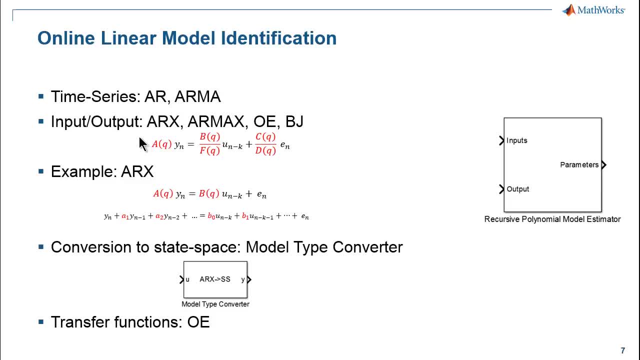 The overall structure of these models look like the equation I have here, where here the A, B, C, D, F polynomials that are in red are functions of the delay operator. Q. yn is the measured output at time n. un-k is the input at time n-k. 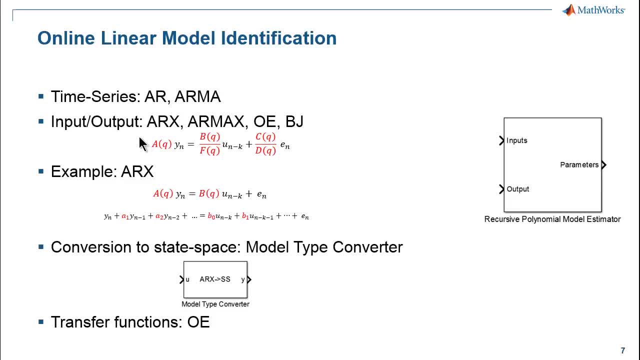 where k represents the time delay And then en is unmeasured disturbance signal. Each one of the model structures I was mentioning estimate a subset of these polynomials and assume that the rest of the polynomials are just one. For instance, the ARX model structure consists of: 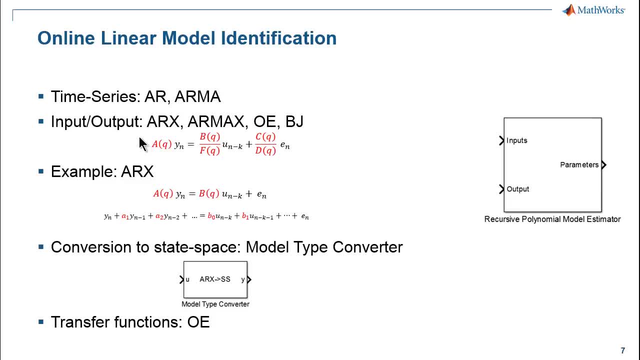 estimating the aq and bq polynomial coefficients. If we look into the equation in detail, what we see here is that the current output, yn, is a function of the past outputs- yn-1,, yn-2, multiplied by some coefficients- a1 and a2- that we will be estimating in the block. 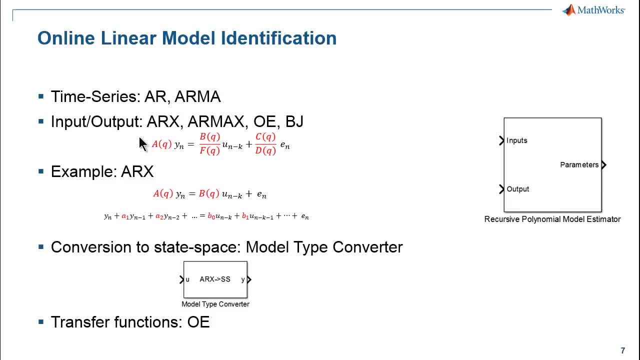 in addition to past values of input signal u, again multiplied with some coefficients we will be estimating plus a noise turn. If these model structures are not very familiar to you, in the system identification toolbox we provide a model type converter which takes these parameters and then converts it to. 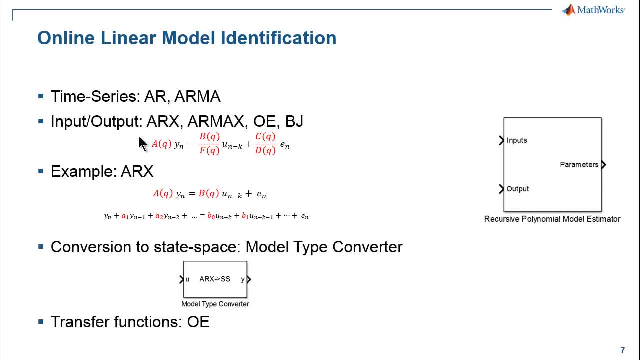 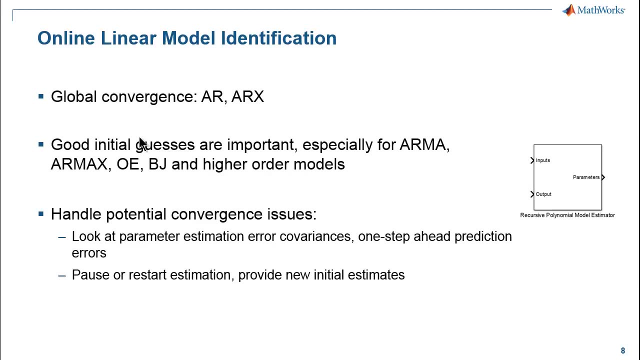 state-space matrices. In addition, the output error model structure, which basically estimates the b and f polynomials here, can be considered as a transfer function estimation. I would like to talk a little bit about the underlying algorithms for the estimation of these model structures. 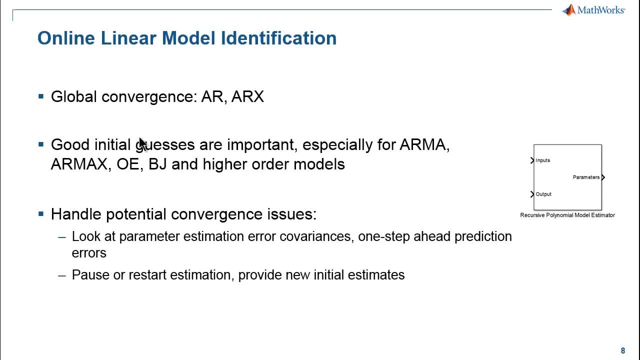 You know, since there are multiple model structures, a natural question is where to start with. On that front, the initial answer would be based on your application. if it's a time series problem or an input-output model kind of problem, it would be AR or ARX. 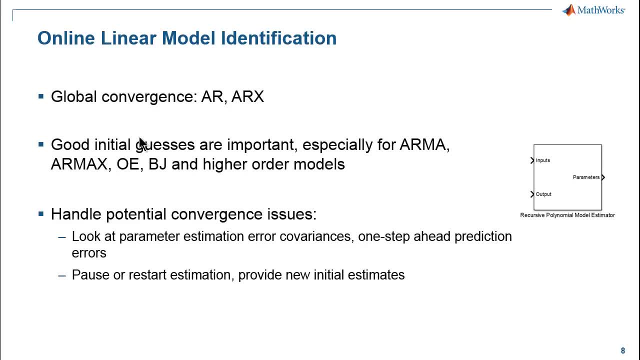 The main reason is that the estimation of these model types, the underlying estimation problem, specifically a recursively squares problem- is a convex problem. That means the algorithms have global convergence. This implies that, regardless of the initial parameter estimates you provide to the block, 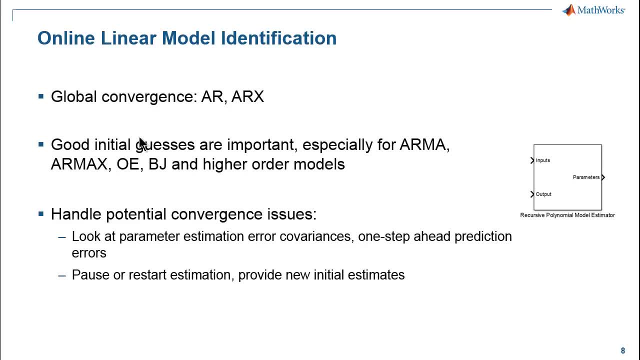 after sufficient time the estimation algorithm will converge to the global optima, So that removes partially the concerns about guessing the initial parameters. The good initial guesses are more important for the other model structures because their estimation is done via a method called recursive parameter error minimization. 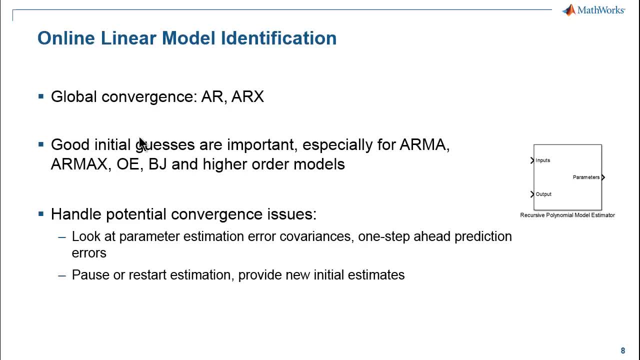 which is not a convex problem. Therefore, where the algorithm converges depends on the initial guesses, And this is even more so important for higher order models. This block provides you a few tools that you can utilize to handle some potential convergence issues online. 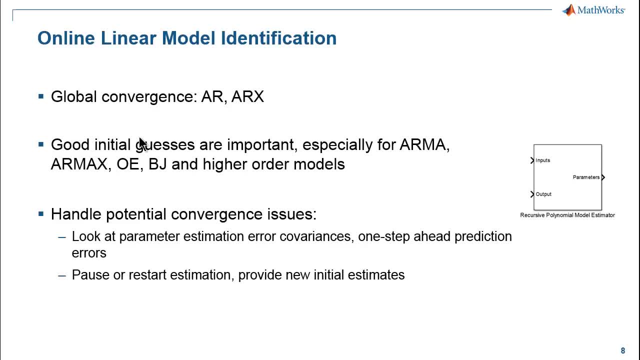 For example, for validation purposes. this block provides you so-called estimation error, covariances, one-step-ahead prediction errors, and I will give you more details about validation in the following slides. In addition, with this block, you can, for instance, pause your estimation. 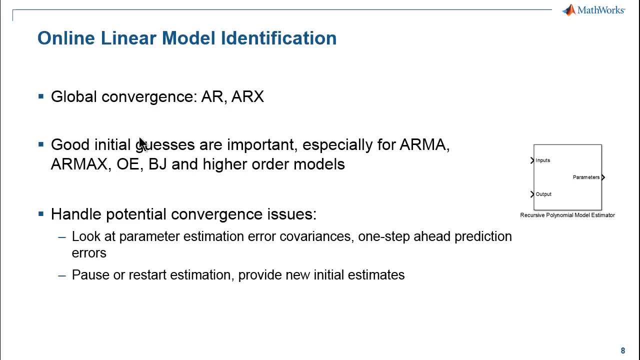 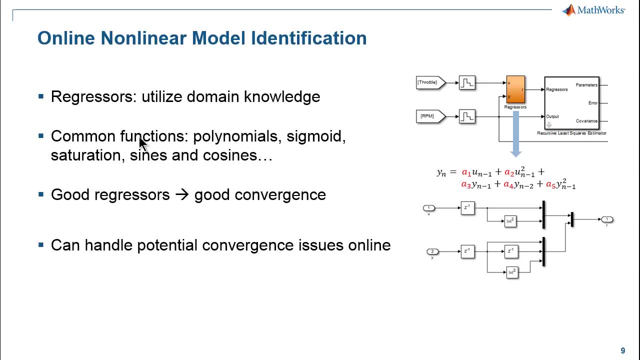 when your input and output measurements are not good enough, or if there is a convergence to a bad set of parameters, you can restart estimation from any point you may want to start from again. Now I will introduce you our second block, namely the recursively squares estimator block. 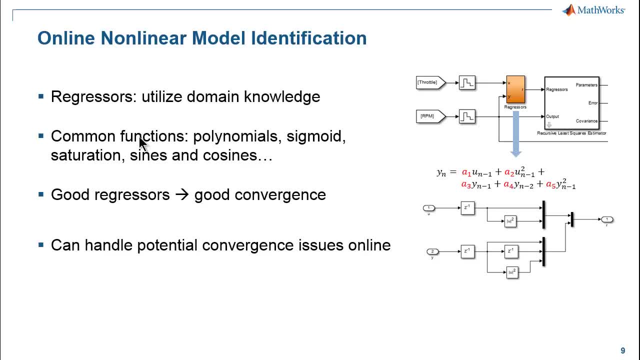 With this block, the structure of the estimated model is more flexible. I have one example on the right where the equation shows the current output. yn is a function of some polynomial terms of the past input and output values. Here on the right-hand side of the equation. 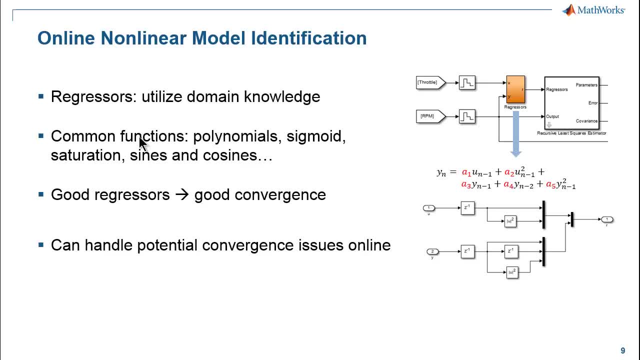 the terms in black are called the regressors and this is what you provide into the block And this is what you would implement here in this block in orange. The parameters in red are estimated by the block. A question is how to pick these regressors. 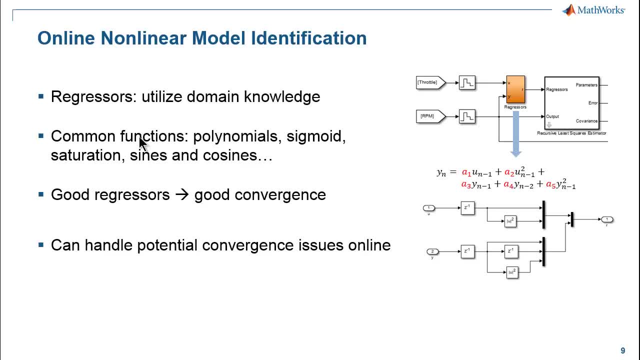 and typically these are done by utilizing your domain knowledge. That being said, there are some common functions that are used pretty frequently. Those are polynomials, sigmoid functions, saturation, sines and cosines. These are pretty good basis functions, As the name of the block implies. 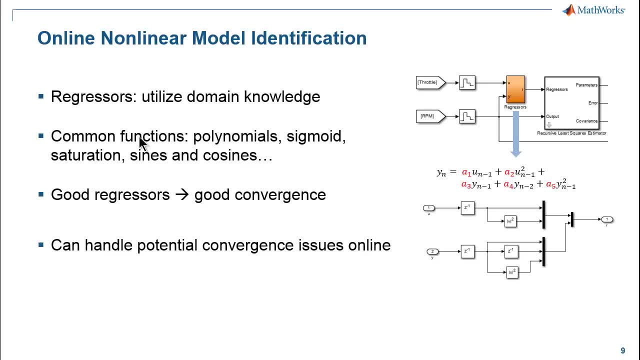 the algorithm here is a recursively squares problem, which means well, it's a convex problem, and if you choose good regressors, that means you will be getting good convergence, Just like the recursive polynomial model estimator block. this block gives you various tools. 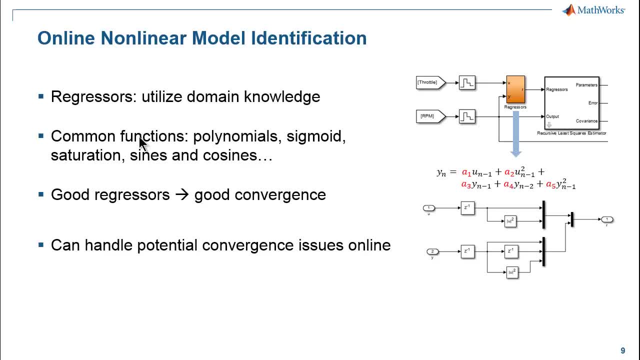 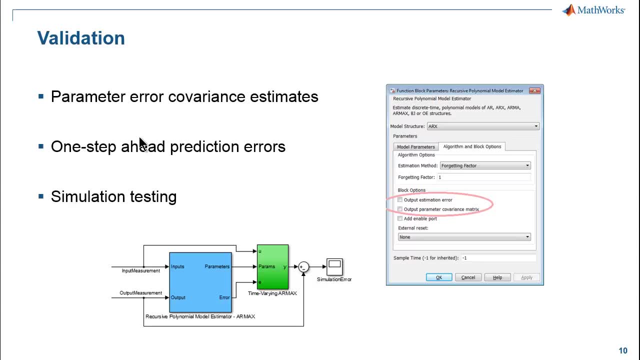 to handle potential convergence issues online. When you are doing online parameter estimation, a natural question is: how reliable are the estimated parameters? I will touch on three ways of looking at this. The first one is so-called parameter error covariance estimates. This is an extra information optionally. 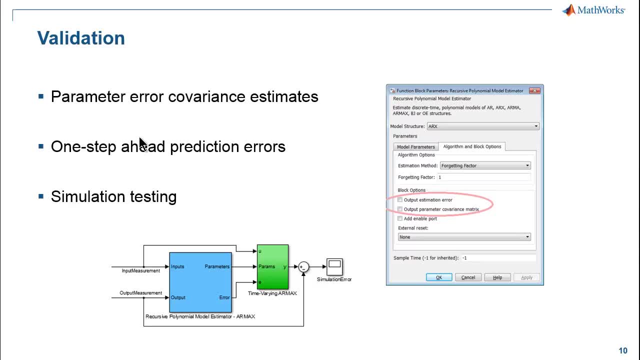 you can get from both of our blocks. To get these you would go to your block dialog and then in the algorithm and block options here I circled in red. these are the optional outputs you can use for further validation Once you check the output parameter. error covariance matrix. 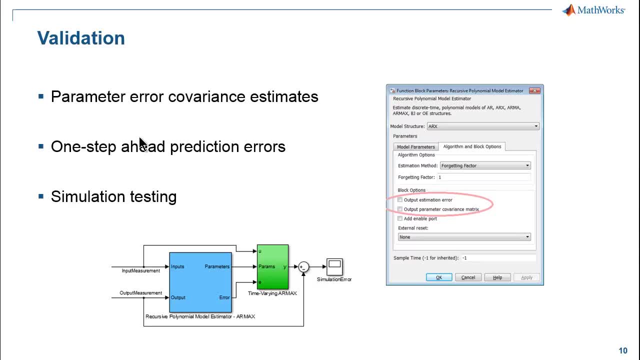 you would be getting this information, which basically tells you how much the block trusts in the estimated parameters. Therefore, the smaller the covariances are, the better. The second thing you can look at is so-called one-step-ahead prediction errors, which you get from the block. 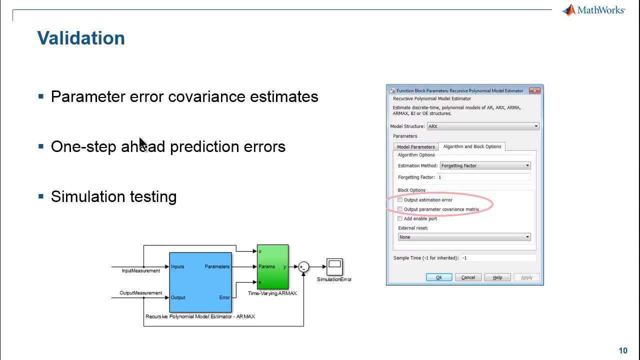 when you check this optional output estimation error checkbox, This represents the error between the blocks: estimate of the system output at the current time step and then the measured one. Ideally this should be small bounded and it should be white, meaning the signal should not be correlated with itself. 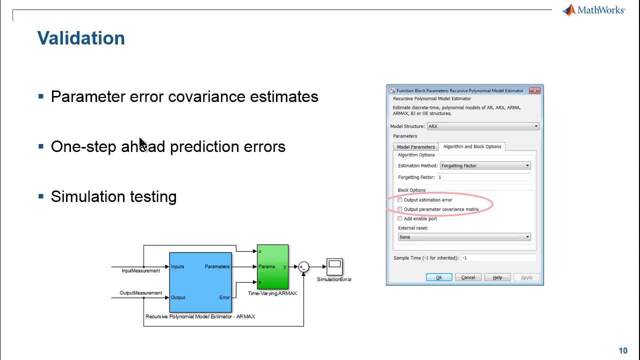 Third way of looking at validation is so-called simulation testing, where I am demonstrating a simple block diagram right below here, where I am taking the input measurements from my system and I am taking the estimated parameters from the online estimation block and then I am just simulating. 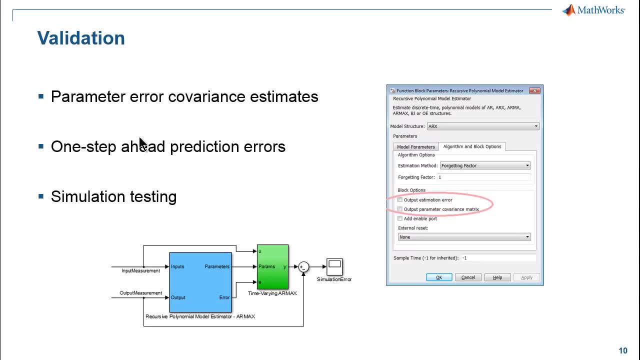 the model forward in time. This gives a more strict validation result compared to the one-step-ahead prediction. errors, and then, in this case again, the error between the output measurement and then the output of the simulated system should be small and bounded. I would like to share just a few. 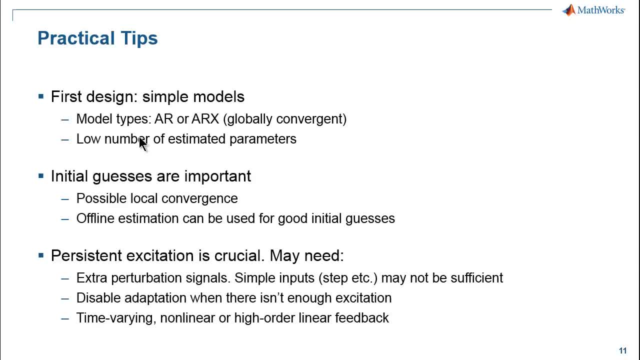 practical tips at this point, When you are doing your first design. keeping it simple is very important In terms of choosing a model structure. if you are estimating a polynomial model, AR and ARX are good choices because these are convex problems and the algorithms are globally convergent. 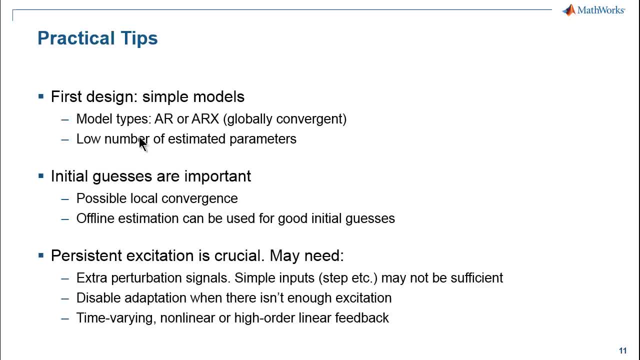 In addition, if you are using the recursively squares block, this is about choosing good regressors. Again, starting simple is a very good idea. The online estimation problem gets much harder when you have a high number of estimated parameters. Keeping this low would be a good idea. 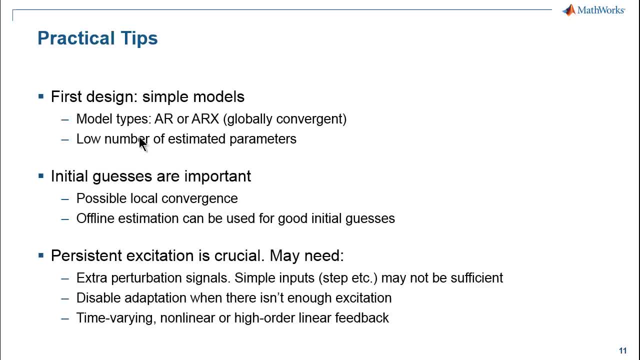 For any other model types, for the polynomial model estimator block, the initial guesses are very important since there is a real chance of convergence to a local optima. At this point, one idea may be if you know the initial state of your system. 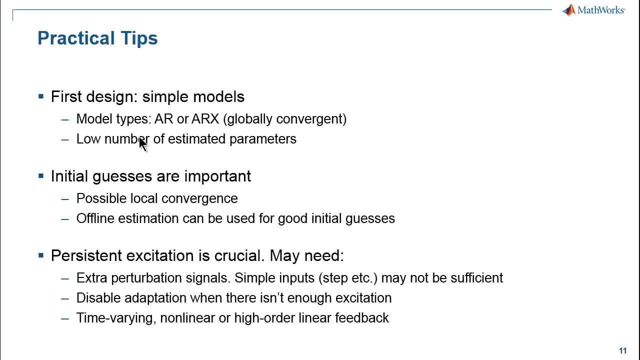 you could utilize the offline estimation capabilities that are available in the system identification toolbox to get a really good set of initial guesses and then let the online parameter estimation work from that point on. In online estimation, so-called persistent excitation is very crucial, which is basically a condition. 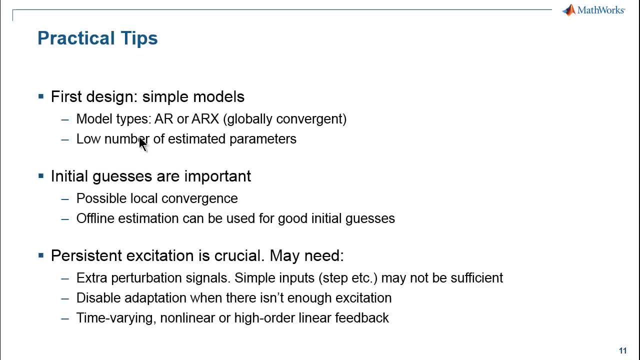 on the inputs to your system. You may have to implement some extra perturbation signals just to have enough information in the input and output signals to be able to identify your model. For example, simple inputs such as step inputs may not be sufficient to identify. 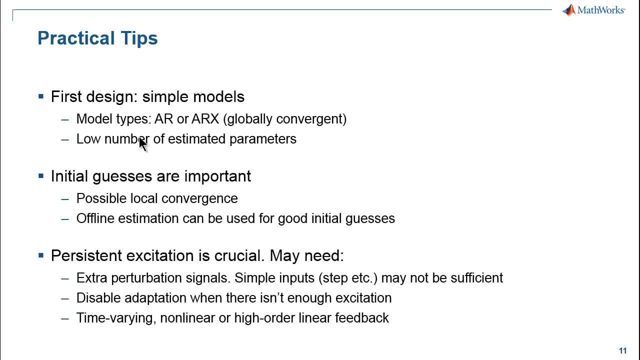 more than one parameters, It's a good rule of thumb to only use good data, so therefore you can or you may need to disable the adaptation when there is not enough excitation in your system. The third point is typically online parameter estimation. 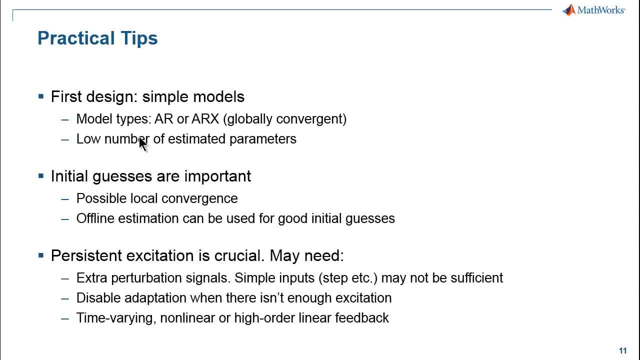 is used in closed-loop systems. Closed-loop systems can introduce some extra problems. Concretely, if you have a simple feedback controller and a simple model, in presence of closed-loop, your controller may make two different systems look the same. Therefore. 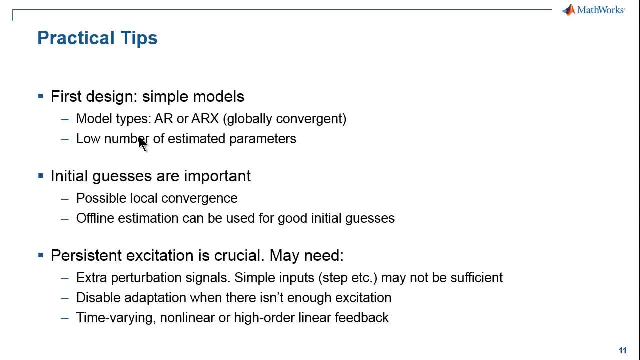 your system may not be identifiable. One way to address that is using a time-varying or a non-linear or a high-order linear feedback controller. Typically, if it's an adaptive controller problem, then you would be already having time-varying or non-linear controllers. 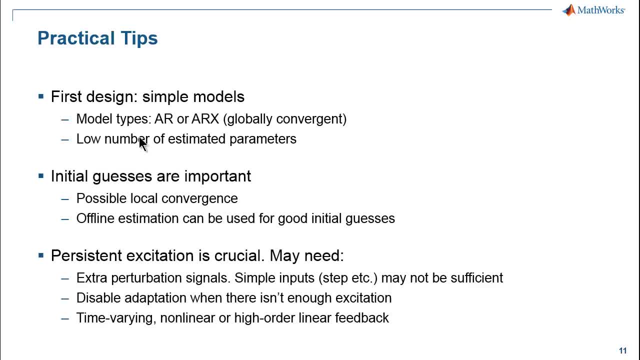 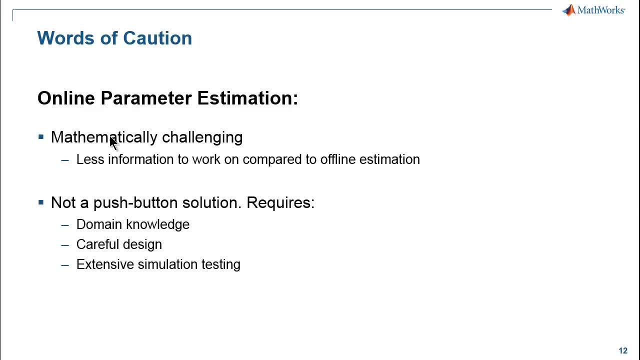 but this is something to keep in mind, especially for fault detection algorithms. I would also like to share a few words of caution at this point. Online parameter estimation is typically mathematically more challenging compared to offline estimation. This is basically because offline estimation has more information to work on. 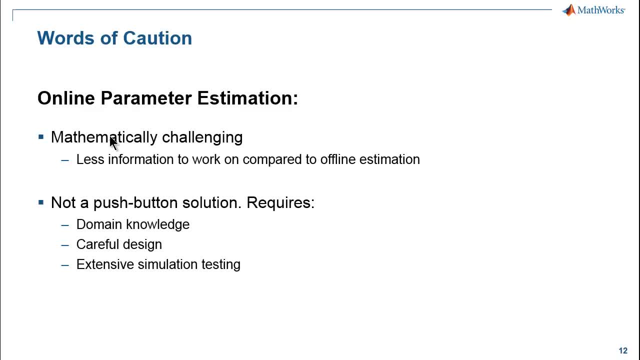 which is all the past inputs and you can work on them all at once, whereas in online parameter estimation, you are working on just your previous estimates and then the recent data. This puts some fundamental constraints on how well you can do in terms of parameter estimation. 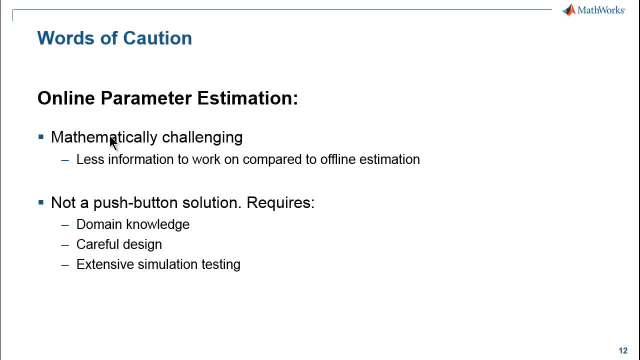 I think the key takeaway point here is: you should be using online parameter estimation only when it's necessary. The second point I would like to say is: this is not a push-button solution. It requires domain knowledge, careful design of various parameters and in terms of the validation. 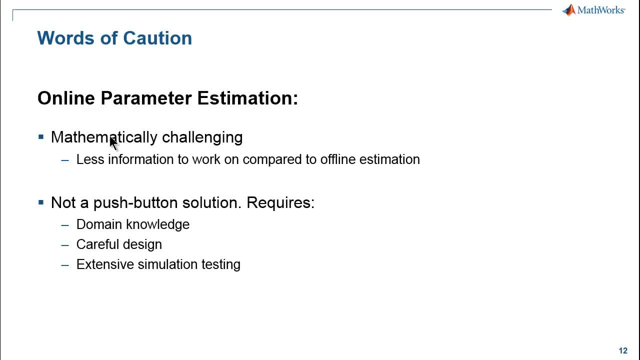 typically you would have to do extensive simulation testing. I would like to say this is a very powerful tool, but it should be used when it's necessary. All the blocks and capabilities I've been introducing to you so far: they support C and C++ code generation. 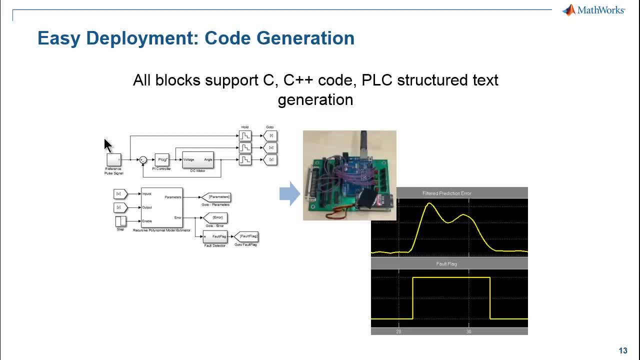 and PLC structured text generation. This is a very straightforward process and it's as simple as hitting one button, and at this point I would like to show you a video demonstrating this capability. In this video, you'll see how to perform online parameter estimation. 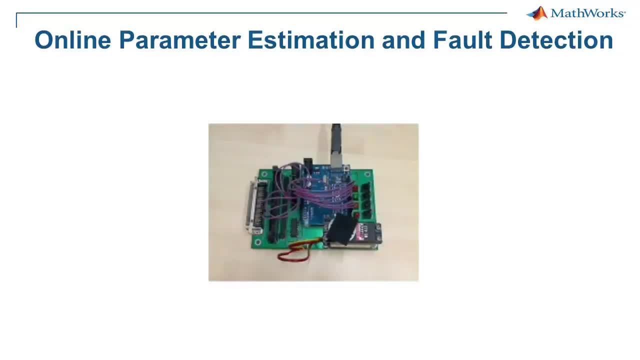 and fault detection using System Identification Toolbox. To demonstrate this, we will be using this hobby DC motor connected to an Arduino Uno board through a driver. The embedded algorithm running on the Arduino Uno tracks the reference angle commanded to the motor. The algorithm also performs. 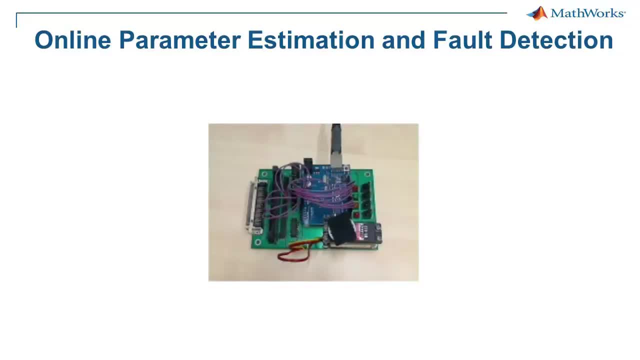 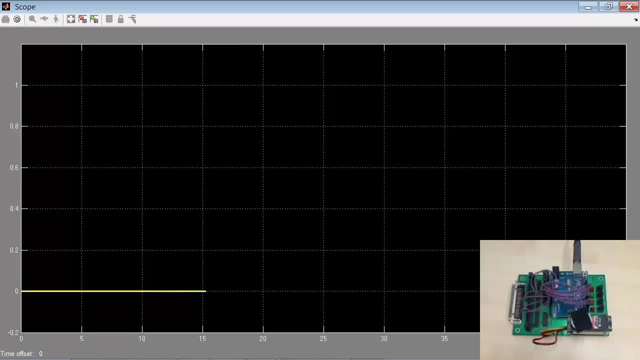 online parameter estimation and fault detection to calculate a fault flag that we see on the scope. During the normal operation of the DC motor, the fault flag is set to zero. However, when we apply a load to the motor, the embedded algorithm quickly determines. 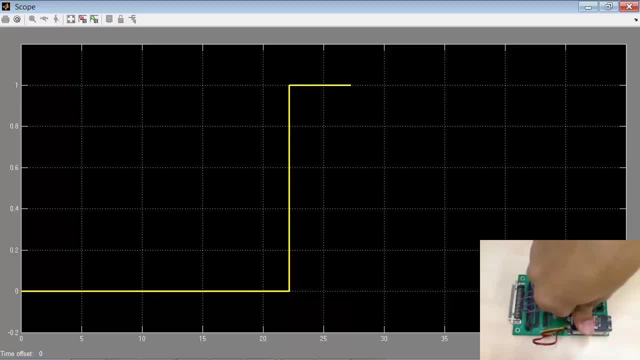 that motor dynamics has changed and sets the fault flag to one. When we remove the load, the algorithm detects that motor dynamics is back to normal and sets the fault flag back to zero. I will emphasize again that the online parameter estimation algorithm is running on the Arduino Uno board. 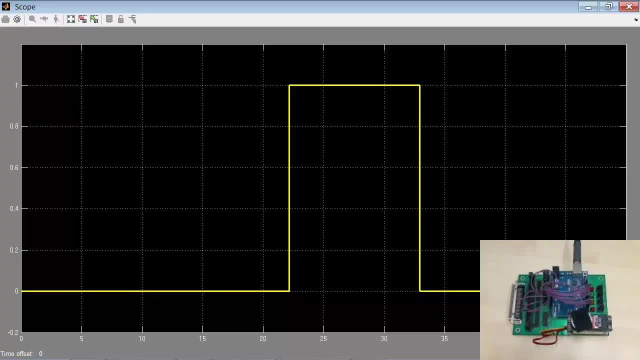 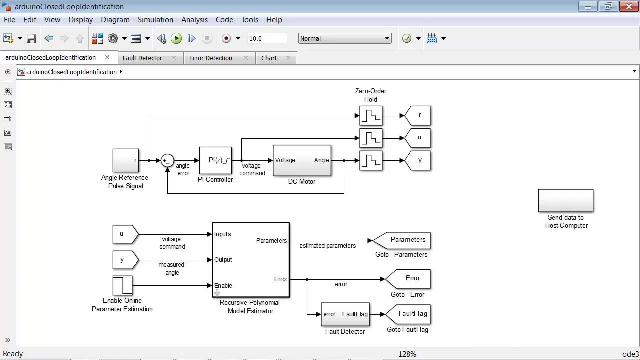 and is detecting changes in motor dynamics as they occur. Let us now take a look at how we implemented this algorithm using Simulink and System Identification Toolbox. We used this Simulink model and automatically generated code from it to program the Arduino Uno. 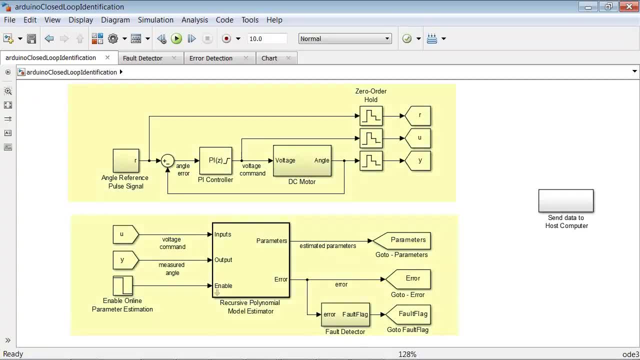 Let us take a closer look at this model. It has two main parts. The first part is a simple PI controller that we tuned for reference tracking. The PI controller takes the angle tracking error and generates voltage commands for the DC motor. The angle reference signal is small enough. 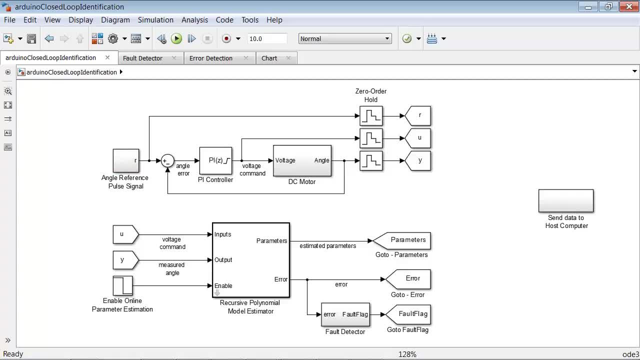 to keep the DC motor within its linear operating conditions. The second part of the model is the online parameter estimation and fault detection algorithm. We provide the voltage command to the motor and the measured motor angle as inputs to the recursive polynomial model estimator block which is present in the System Identification Toolbox. 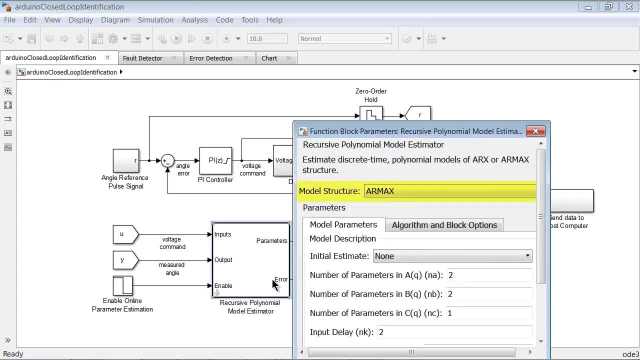 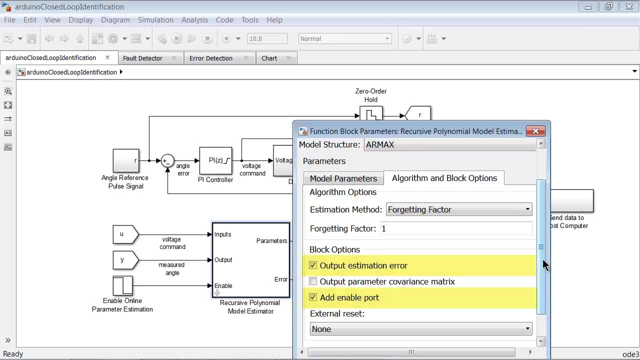 We configured this block to estimate a polynomial model of the DC motor with an RMAC structure, ie autoregressive moving average model with exogenous inputs. We also added the error port and the enable port by selecting the appropriate options in this block. 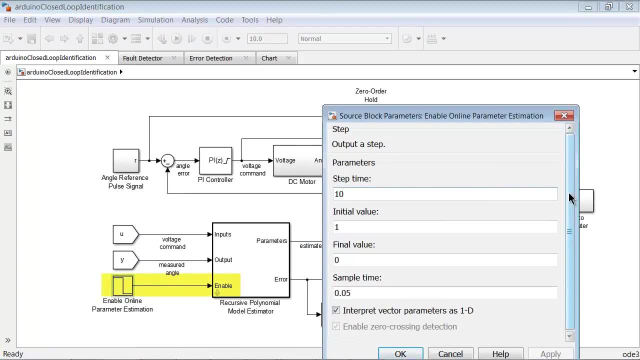 We use the enable port to perform online parameter estimation for the first 10 seconds of the experiment. This enables the estimated model parameters to converge to steady-state values. After 10 seconds, we disable online parameter estimation and the block holds the estimated parameter values constant. 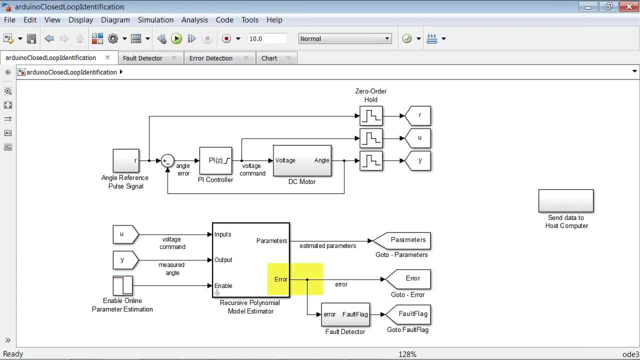 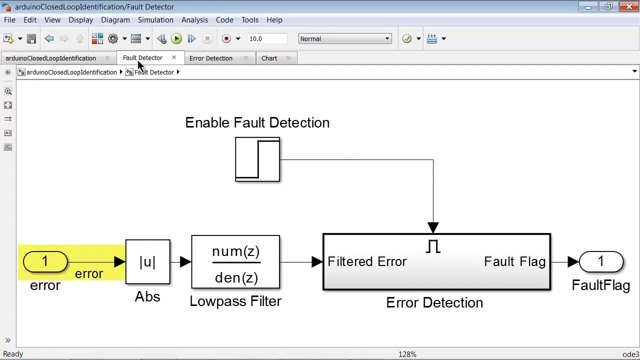 This will help us detect changes in motor dynamics. The error port outputs a step-ahead prediction error, ie the difference between the measured motor angle at the current time and its estimate from the block. We pass this prediction error through a low-pass filter. 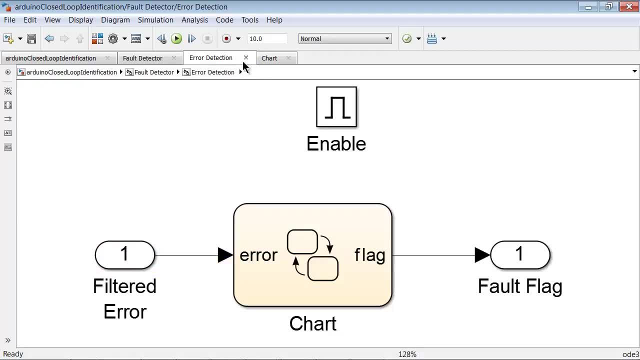 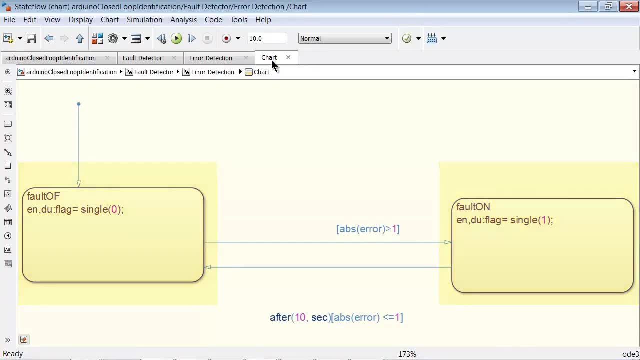 This filtered signal is the input to the fault detection algorithm, which is implemented using a simple two-state state flow chart. The state flow chart sets the fault flag to 1 and the filtered error is greater than a threshold and resets the fault flag back to 0 after the filtered error. 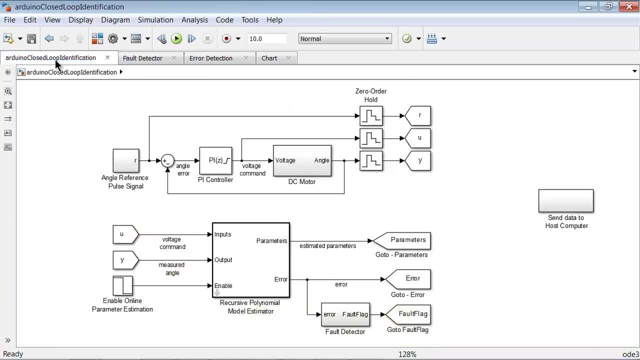 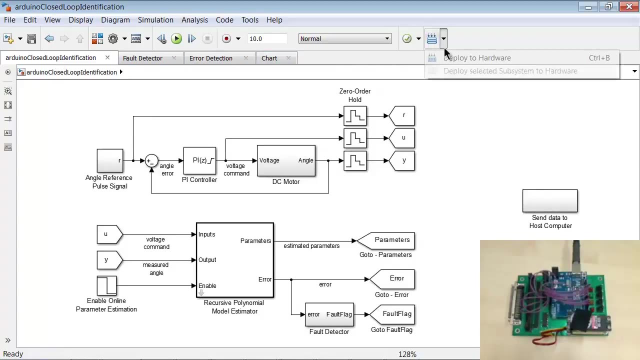 is less than the threshold for 10 seconds. The model also sends signals of interest, ie prediction error and the fault flag, to the host computer, so that we can observe the experiment results in real-time on the host machine. The model also sends signals of interest. 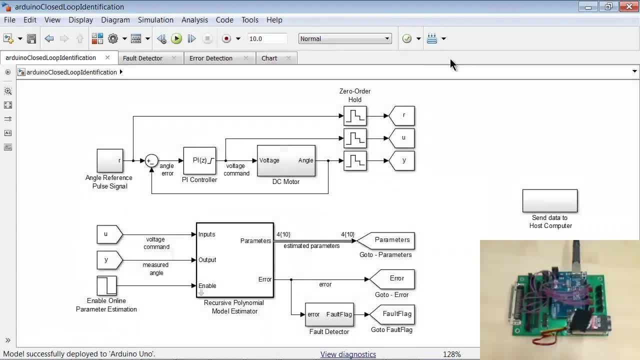 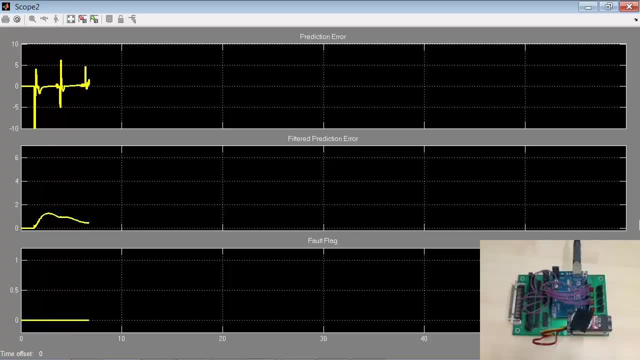 and loads the generated code onto the Arduino Uno. Once this is complete, let us start our experiment. The scope here shows the one-step-ahead prediction error, its low-pass filtered version and the fault detection flag By the time-reducible adaptation at 10 seconds. 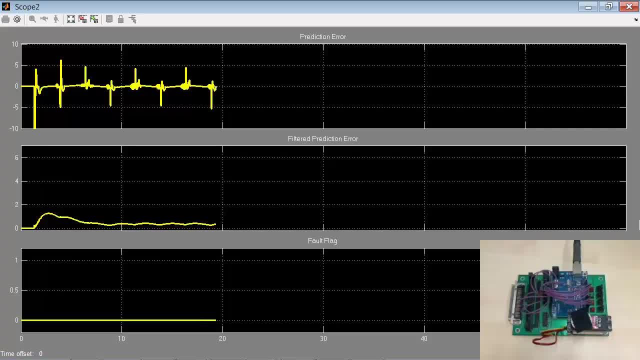 the parameter estimation converges and the prediction error is close to 0. The prediction error shoots up and the fault flag gets set. When the load is removed, the prediction error falls, causing the fault flag to reset to 0.. To summarize, in this video we showed: 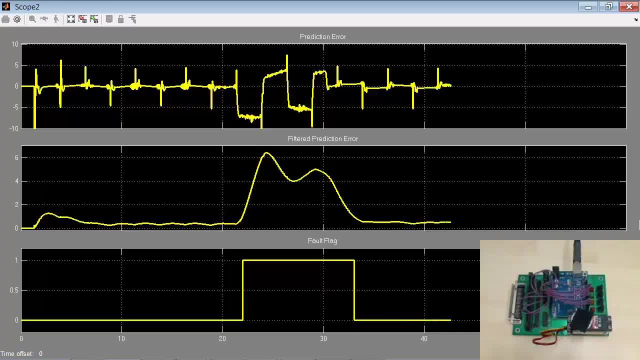 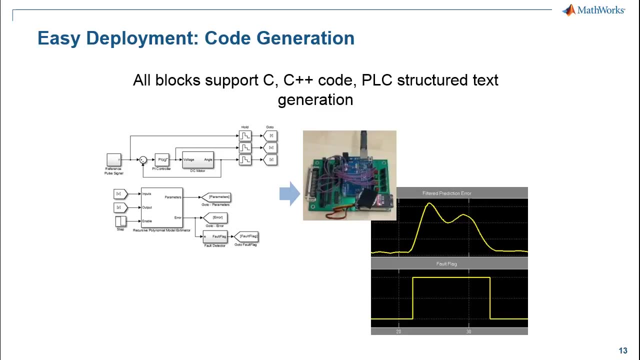 how to use System Identification Toolbox to implement online parameter estimation and fault detection on an embedded processor. This concludes the video. At this point, I will hand over the presentation to Arkady Turevsky. Thanks a lot, Arda. So let me try to summarize. 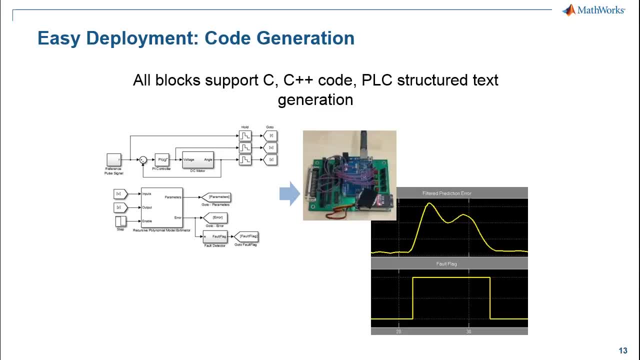 what we have just seen in the presentation that Arda delivered and in the video that he played. So Arda talked about the capabilities recently introduced in System Identification Toolbox for doing online parameter estimation. He showed you principally two different ways to do it: One using the black box approach. 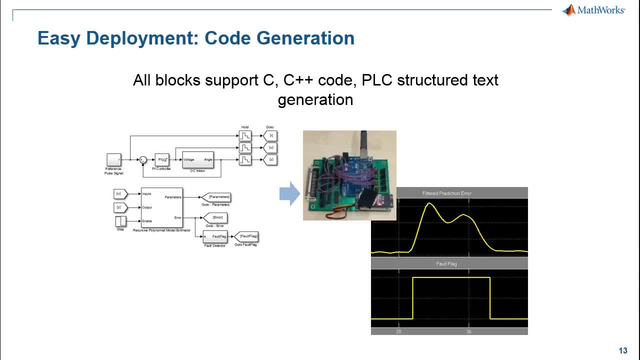 where you estimate a polynomial model that you can then convert to a state space model. This is the approach that you can take if you don't know anything about the physics of your system, And another approach, another block that he showed you that lets you estimate. 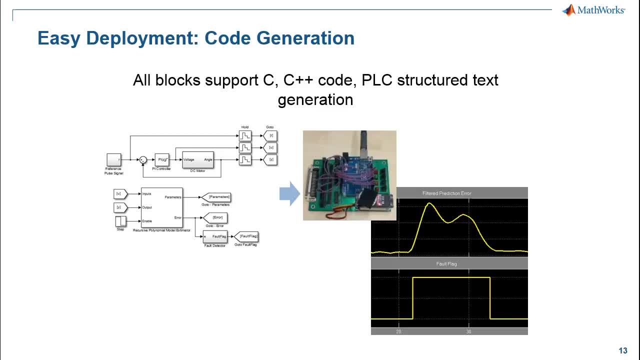 linear coefficients of regressors. So this approach lets you specify regressors that describe the physics of your system. So that approach is more suitable if you have some understanding about the physics of your system. But the bottom line is that there are blocks that you can use. 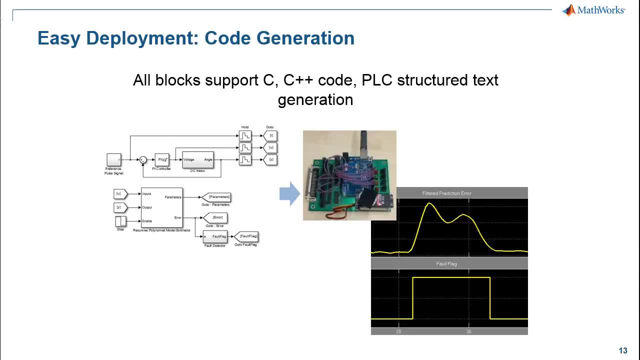 straight from System Identification Toolbox to perform online parameter estimation. You have to know what you are doing, of course. to use these blocks properly, You have to test them in simulation to make sure that they will give you the results that you are expecting. 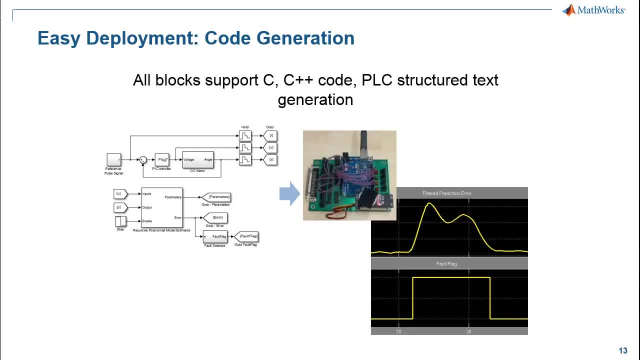 But we have extensive documentation on how to use those And, as we just saw in the video, once you test those blocks in a model, you can deploy the algorithm to an embedded processor by using automatic code generation, because this online parameter estimation blocks support deployment through automatic code generation. 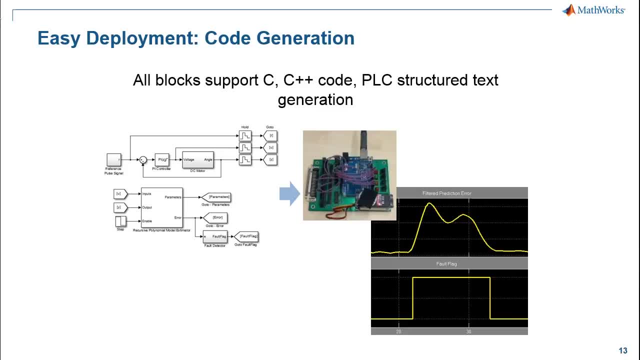 In this particular video, our colleague Karthik showed you how you can deploy online parameter estimation algorithm to an Arduino Uno, Which is a pretty baseline processor in terms of processing power. So this algorithm that we provide for online parameter estimation are not computationally very heavy. 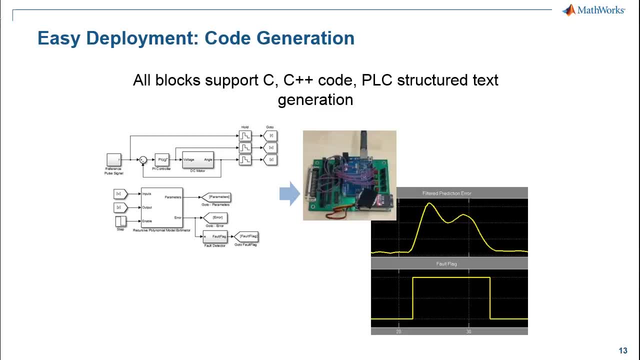 and can be deployed successfully to processors with low throughput and available memory. Now let's move on to the second part of our discussion And, as I said in the beginning, the second part of the discussion is about adaptive control law. So, again, if you look at the block diagram, 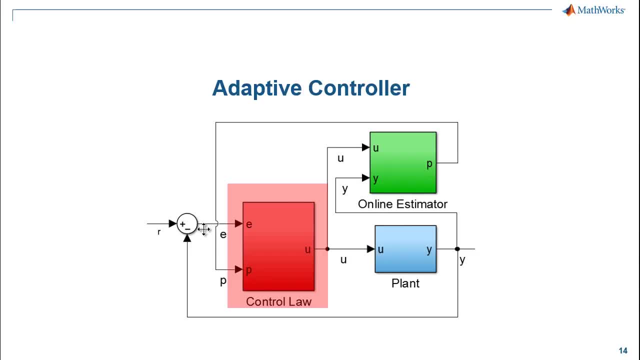 that shows the principal elements of an adaptive controller. now we'll start talking about a control law that can take the parameters estimated by an online estimator and adjust for changes in plan dynamics accordingly. To talk to us about this section, I'll invite my colleague Rong Cheng. 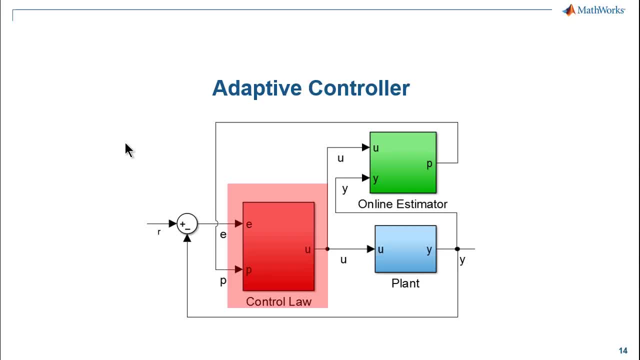 Rong. Thanks, Akadi. As we mentioned before, you can use online estimation techniques such as full diagnosis or parameter estimation, And adaptive control is definitely one of the major areas that you can use online estimation techniques that my colleague Ada just introduced. 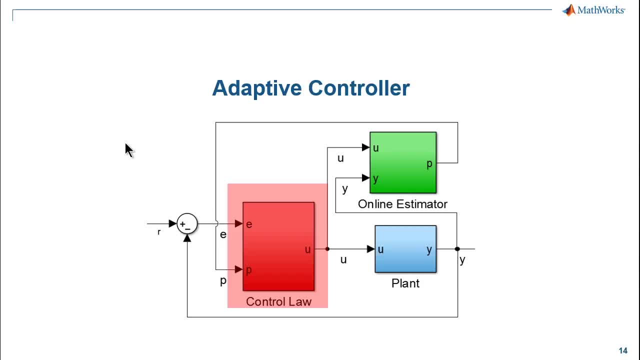 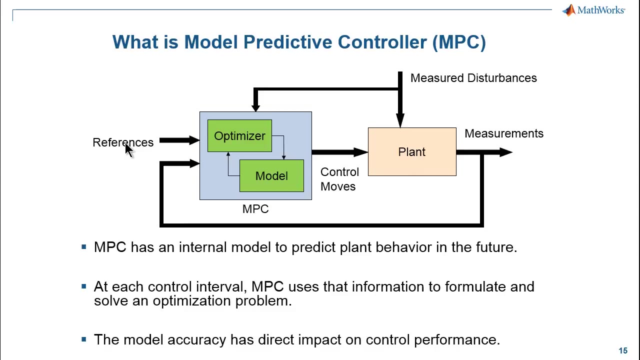 So in the next few minutes I will demonstrate how to use online estimation techniques together with a model predictive controller to control a nonlinear plant. So before I talk about detail about the adaptive MPC, let me first just walk you through quickly about what is the model predictive controller. 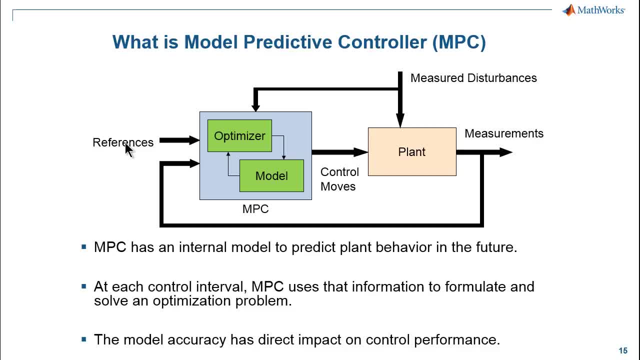 MPC is, in case some of you are not familiar with this particular control technique. So the major difference between the MPC and other control techniques, such as PID and LQR, is that the MPC control itself has an internal plant model to predict the future plant behavior. 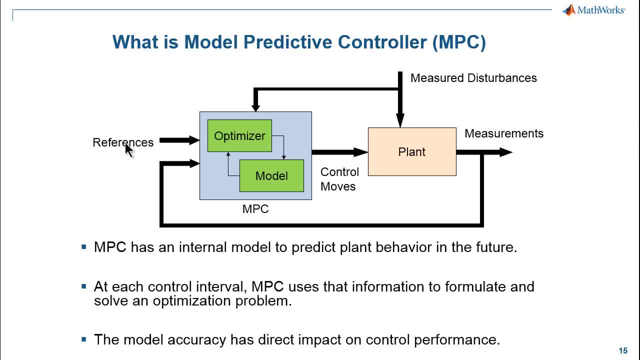 And with that information, MPC will formulate and solve an optimization problem online at each control interval. So, of course, because it has an internal plant model, its accuracy plays a very important role with respect to your controller performance and robustness. So if your plant 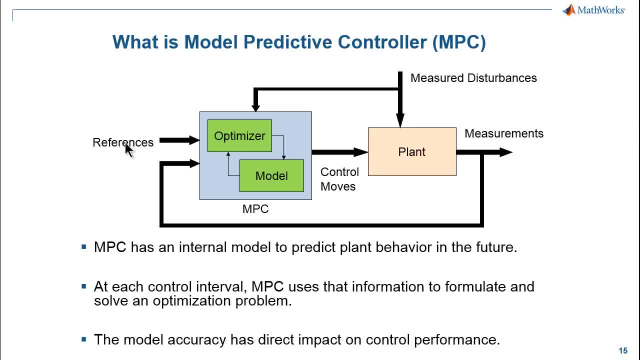 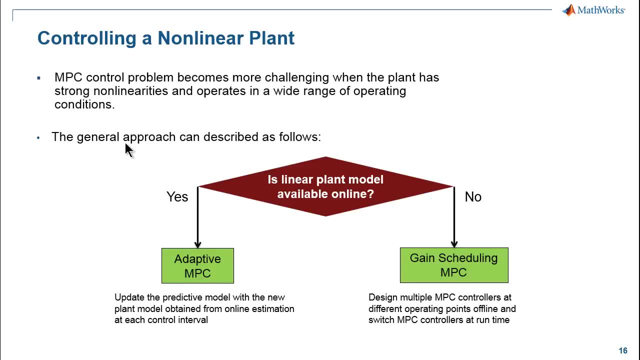 doesn't have strong nonlinearity or doesn't have a very wide range operating point, then usually you can implement a single model predictive controller. that gives you pretty good control, performance and robustness. For example, in this continuous stirred tank reactor it operates. 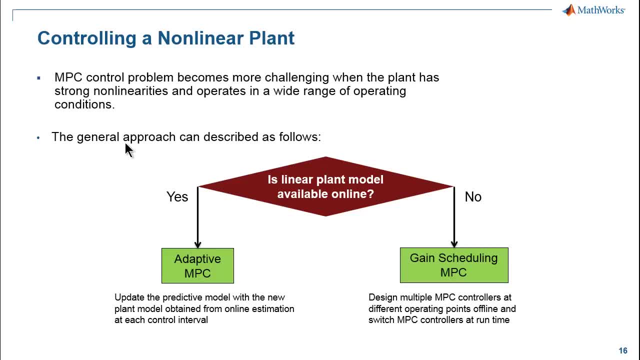 within a wide range of operating points and it has a strong nonlinearity. In this particular case, the plant becomes unstable during the transition. So that gives you a hint that a single MPC which you designed at each operating point probably won't work during the transition. 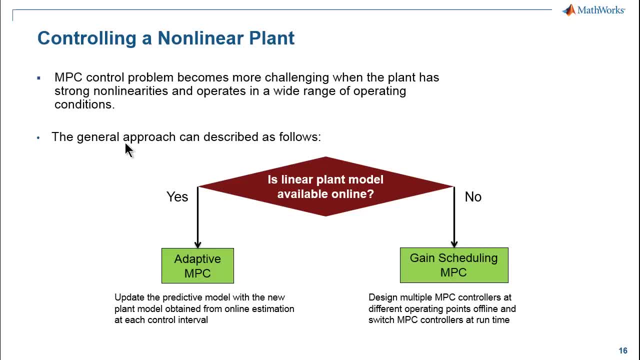 That's exactly as my colleague Akadi already showed you at the beginning of the presentation. So one solution, a general solution, to solve this nonlinear control problem is to use an adaptive controller. So let's look at the way how you can implement. So if you do not, 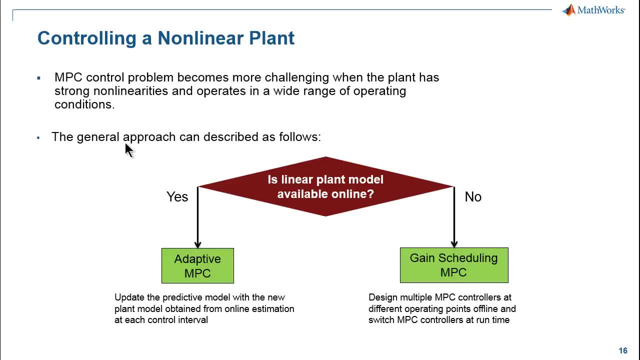 have the ability to obtain a linear plant model online, then you basically can use the gain scheduling technology to solve this nonlinear control problem, in the sense that you can obtain multiple linear plants at different operating points offline and design multiple MPC controllers for each of these operating points. 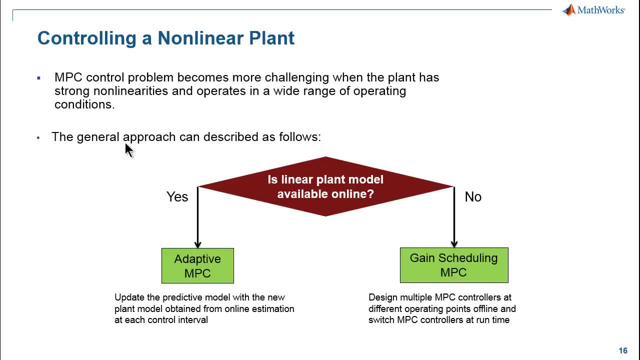 And then when you implement these MPC controllers and depending on where your operating point is. but assumes that now you have the ability to obtain a linear plant model online, for example, you are using the online estimation capability provided by SystemID toolbox, then actually you could use it together. 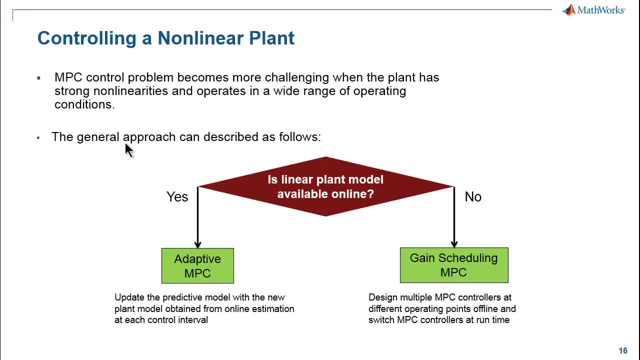 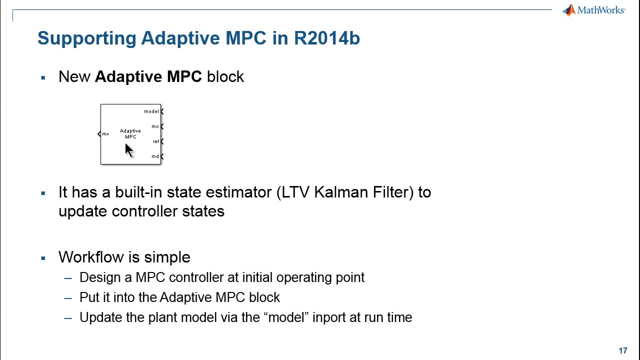 with our MPC block to implement adaptive MPC control scheme in our Simulink environment. So in the rest of my presentation we will cover how you can do it to control this nonlinear CSTR plant. So in 2014B, MPC toolbox has a major 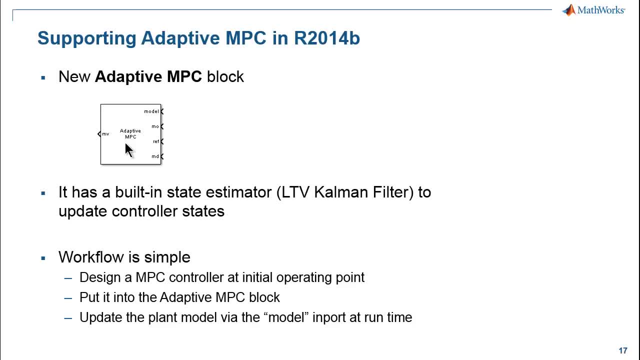 release. There are many new features available, but one of them is the new adaptive MPC block. So from the block diagram you can see that now the MPC block accepts online model update from your signals and then it will use that updated information to predict the plant. 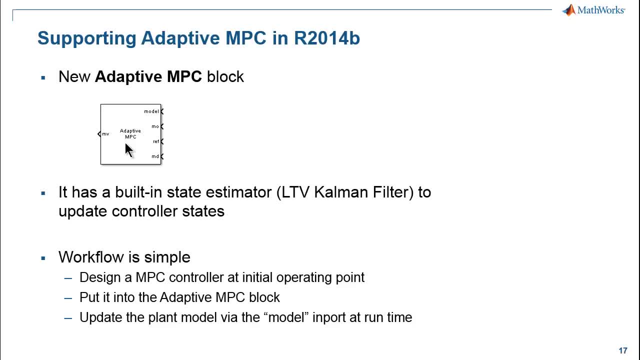 behavior in the future. So the workflow is really simple here. You can basically design an initial MPC controller offline and then you put it into adaptive MPC, So when your plant is running, and then you can just keep updating your plant model through this model import at runtime and so 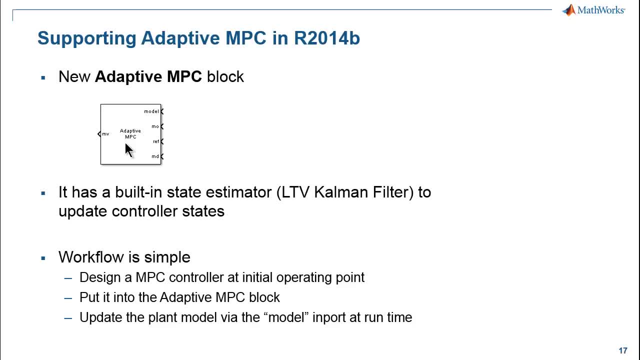 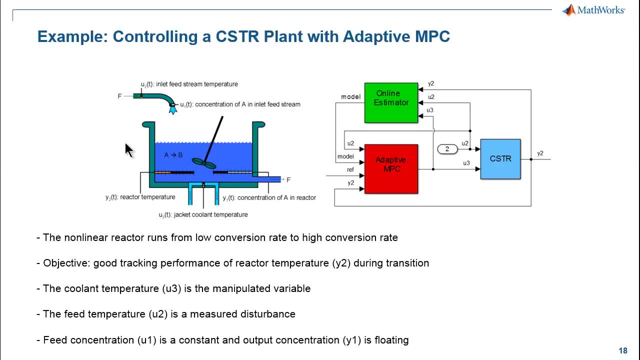 the model could come from an online estimation block, So let's look at how we do that in this particular application. So let's talk a little bit more about the control objectives here. So the goal of this application is to achieve a good tracking performance of 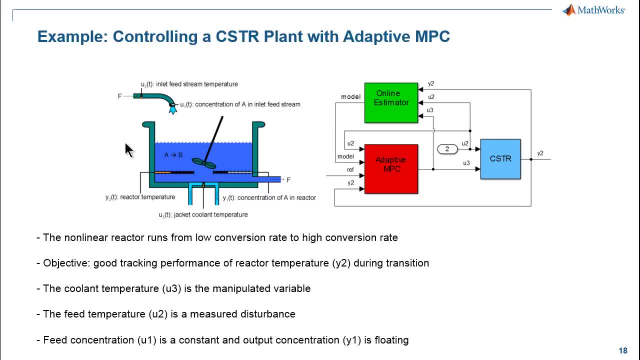 the react temperature, So during the transition period. so the temperature, react temperature profile go from the lower to higher in a linear fashion. So the goal is to make sure the real temperature will follow as close as possible to the profile. So the manipulate variable here is the coolant. 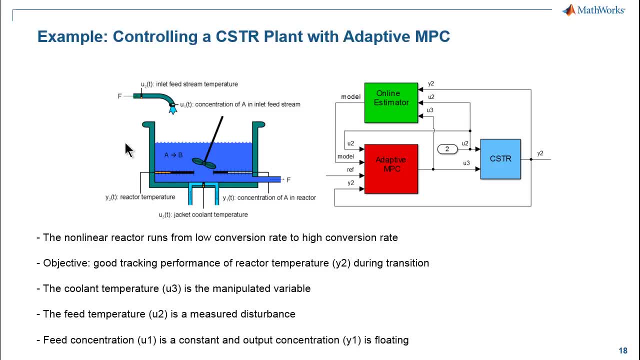 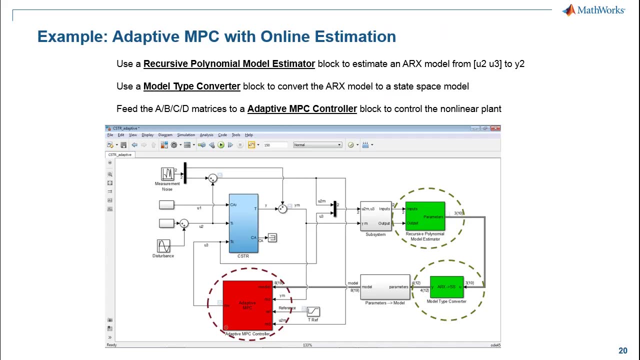 temperature and the feed temperature here is used as the measure. disturbance. Our MPC block will use a feed forward control to make sure it will handle this feed temperature disturbance nicely. Now let's look at how we implement the adaptive MPC scheme in our simulink model. So 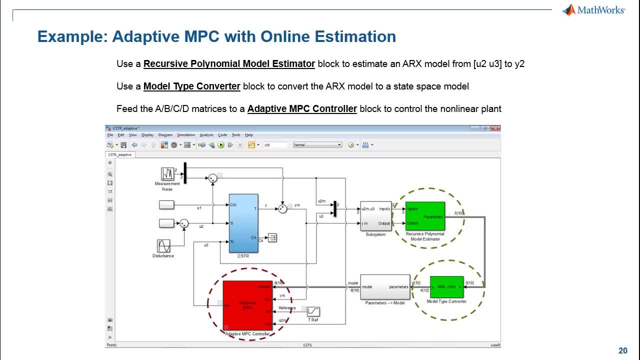 I would like to bring to your attention the three blocks we use here. So for this particular MPC controller, the internal plant model has two inputs and one output, as we mentioned before. So here you can see we use a recursive polynomial model estimator block to: 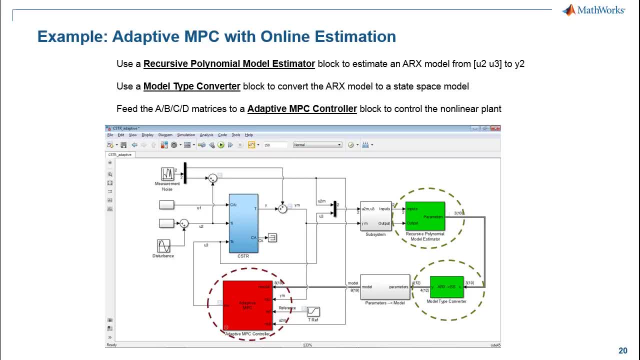 estimate an ARX model for these two inputs and one output. So after we get the polynomial parameters we will feed them into a model type converter block which essentially converts the ARX model to a state space model which is required by the MPC block. 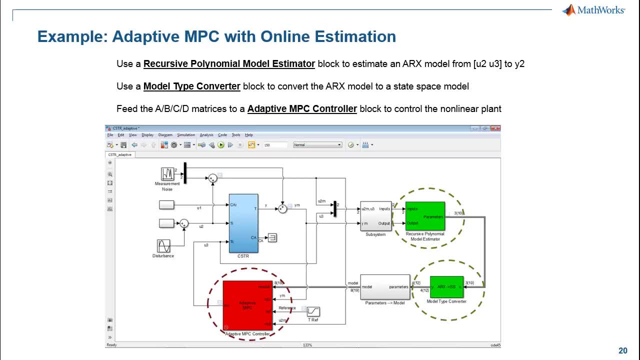 And after you feed the ABCD matrices into the adaptive MPC block to its first input port, then the controller will know what is the current plant model is and will use it in real time to update plant information and to implement the adaptive control part. So this is how. 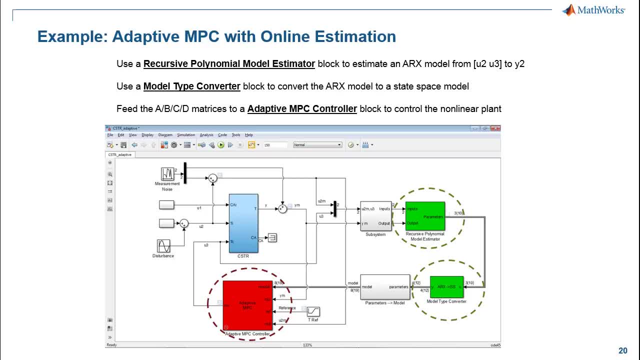 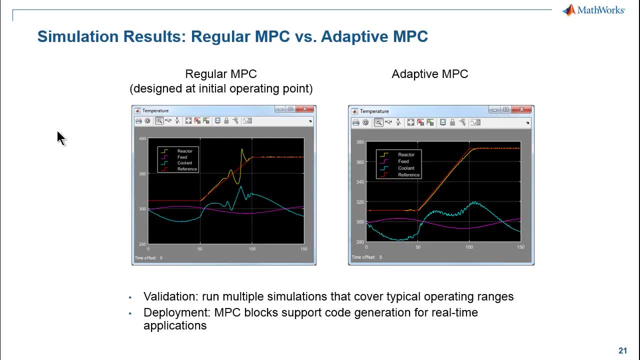 we implemented adaptive control in our simulink model, So let's look at the simulation results. So we would like to compare the results between a single MPC controller and the adaptive MPC controller. On the left side you can see that if you use a single, 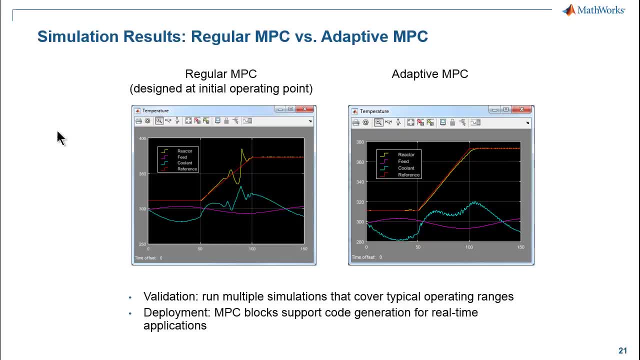 MPC, which is designed at the initial operating point, the tracking performance is really bad because when the plant is transitioning through the unstable mode, the temperature swings wildly and the tracking performance is really not acceptable. But if we use adaptive MPC and because we have the correct, 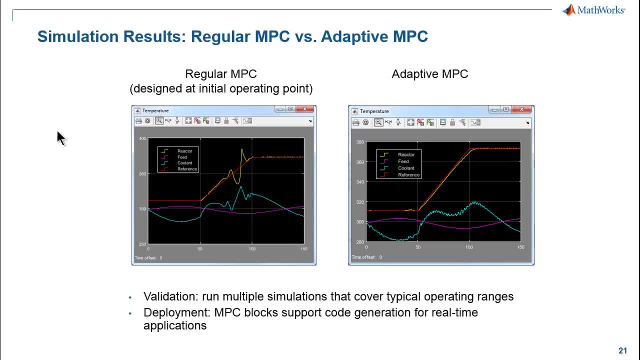 plant model during the transition. the MPC controller does a much better job to predict the future plant behavior and then, in that sense, give a much better tracking performance. So, as we mentioned before, we always recommend people to run multiple simulations that should cover a typical operating. 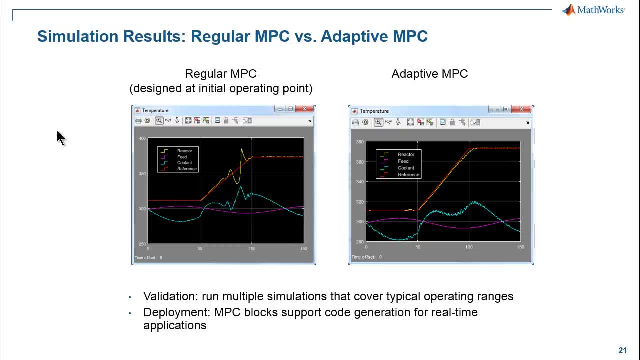 range for your nonlinear plant and with the typical setpoint, changes or disturbance signals you expect. So with multiple simulations you have more confidence that your adaptive controller will work at any operating points that you expect your plant will run under. So in the end you can. 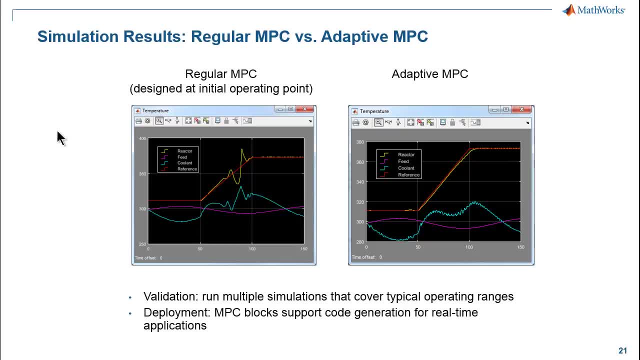 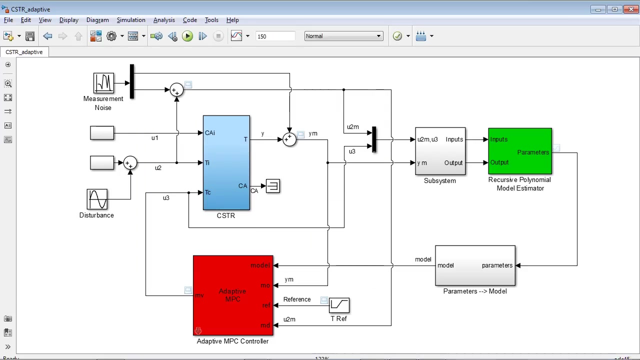 basically deploy your MPC blocks together with online estimation blocks through our simulation coder products and then use them in the real-time application. So before I hand the presentation to Akadi, I would like to show you some parameters we used in both estimation and MPC controllers. So 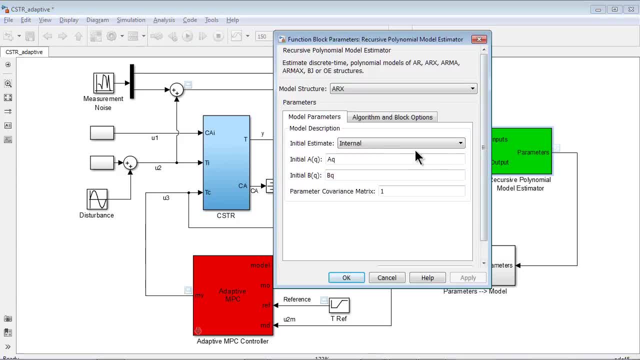 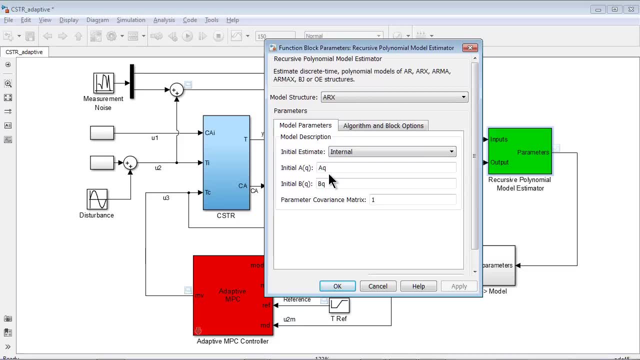 if you look at the recursive polynomial model estimator block, so the initial polynomial coefficients you use here actually derived from transfer function plant model you obtained when you designed initial controller, initial MPC controller. here And in the algorithm part we used a common filter estimation method and the noise 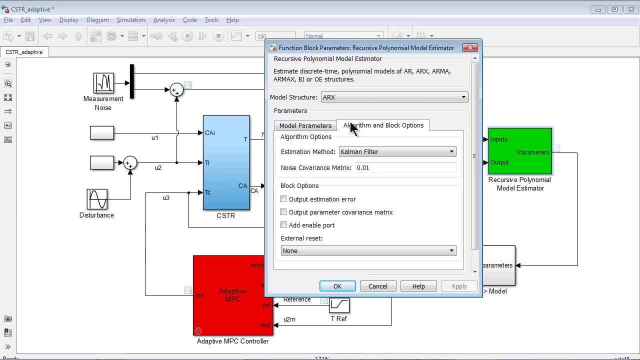 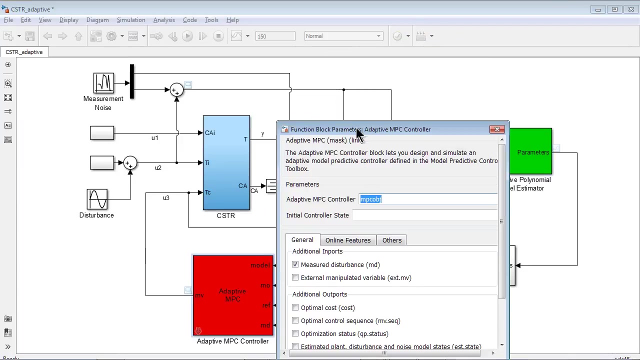 covariance matrix is 0.01.. So, as Ada already mentioned, you need to play with those tuning parameters to make sure that you have a quick and robust convergence during the runtime for the model estimation part. So then let's look at the adaptive MPC blocks. You can 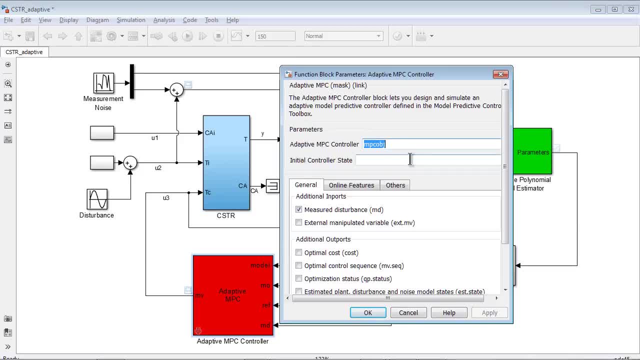 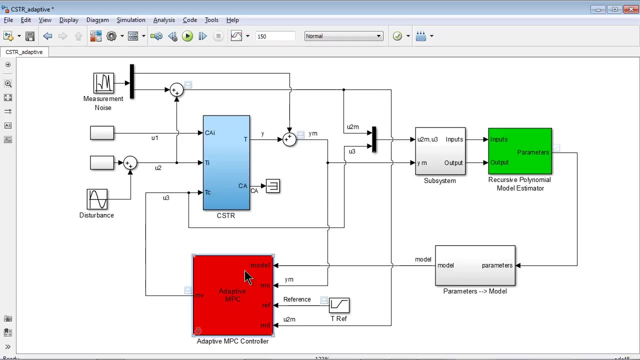 see in this block. we put the MPC controller object there. This is the one you designed at initial operating point. You just enable the measure of disturbance comes in and that's all you need to do, And then the plant will be supplied. model will be supplied. 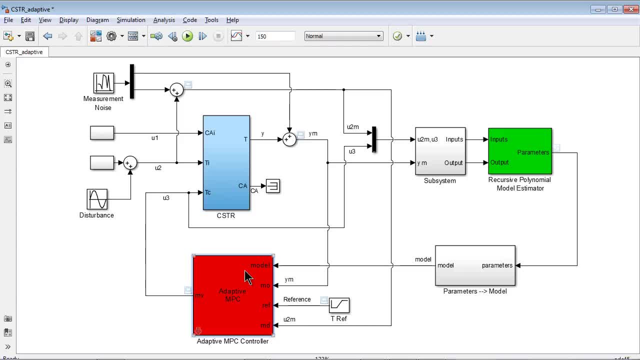 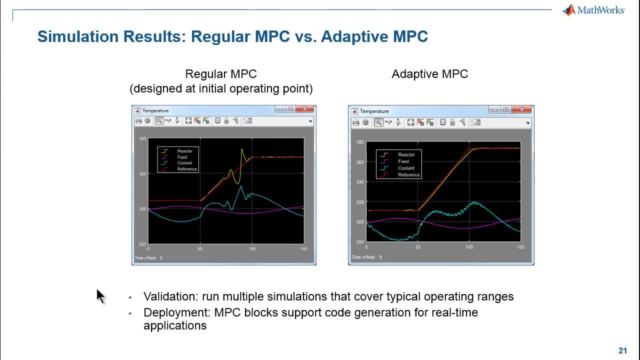 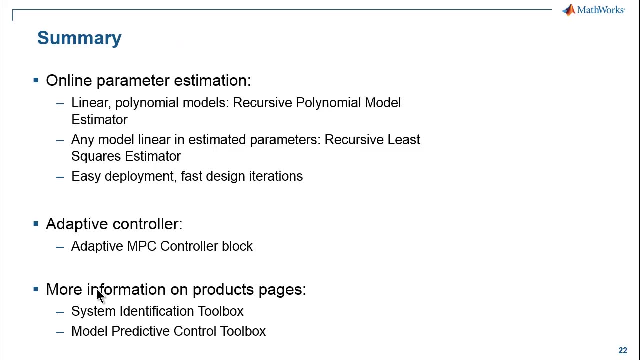 through the first input to the MPC block. With that, I will hand the presentation to my colleague Akadi. Thank you, Rong. So let me summarize what we have seen and heard today. We showed you capabilities currently shipping in our products. System Identification Toolbox. 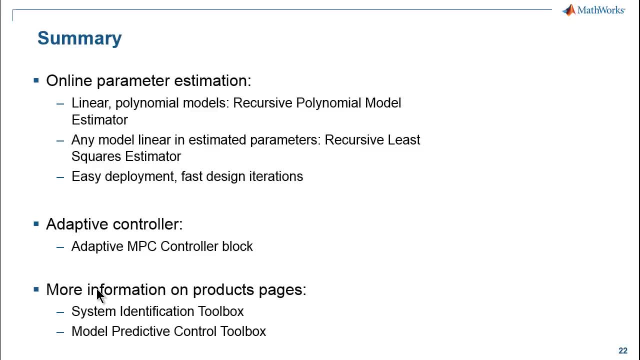 and Model Predictive Control Toolbox for designing, simulating and implementing adaptive controllers. We provide online parameter estimation capabilities in System Identification Toolbox that let you estimate model parameters online using either black box approach or an approach where you know a little bit more about systems physics. 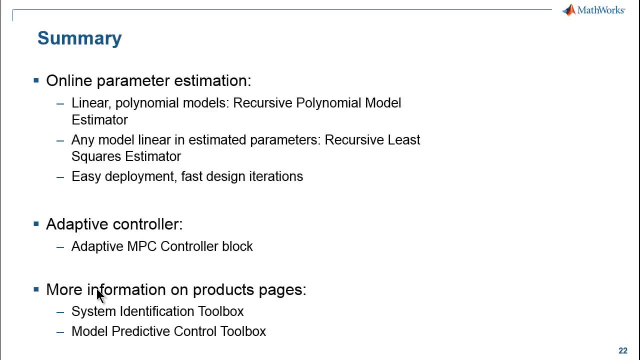 You can use these capabilities for adaptive control or for online fault detection. We provide an out-of-the-box adaptive MPC controller block in Model Predictive Control Toolbox. You can take parameters- plant parameters estimated using online parameter estimation capabilities in System Identification Toolbox and supply them to an adaptive. 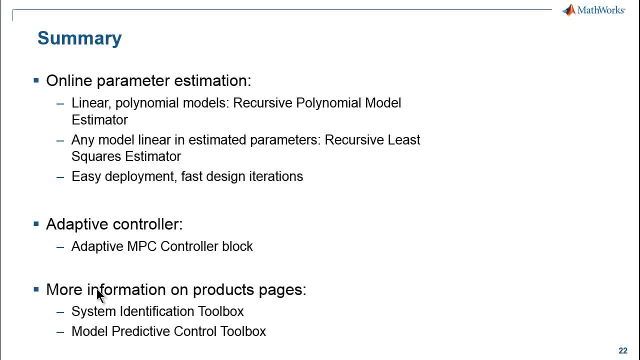 MPC controller. This lets you estimate plant parameters as plant dynamics is changing and adjust controller behavior dynamically during runtime to account for the changes in plant dynamics. We have more information and examples on product pages, So I encourage you to visit System Identification Toolbox page and Model Predictive Control Toolbox. 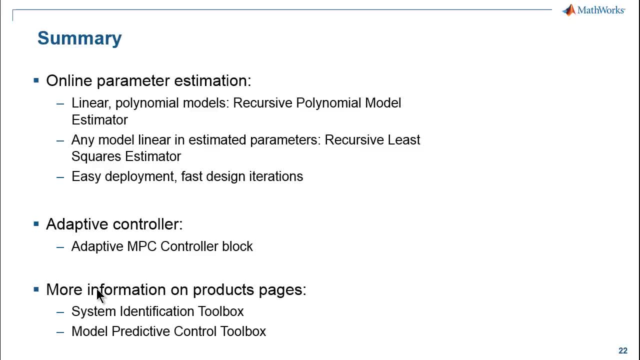 page to learn more. As was mentioned multiple times, this approach requires thorough validation by running a lot of simulations and testing all possible scenarios through simulation. But both blocks for online parameter estimation and the block for adaptive MPC controller support implementation using automatic code generation. so 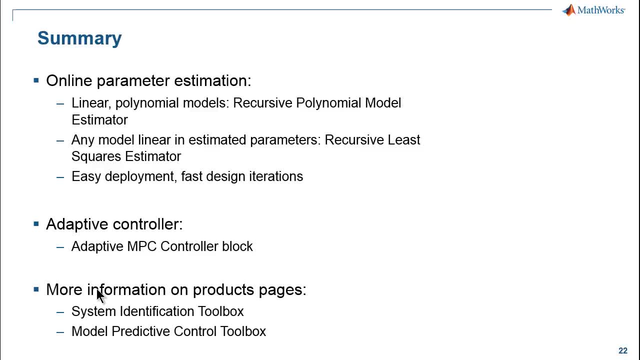 you can implement adaptive control algorithms on your embedded microprocessor. We hope that you found this webinar interesting. Thank you very much for attending this webinar.